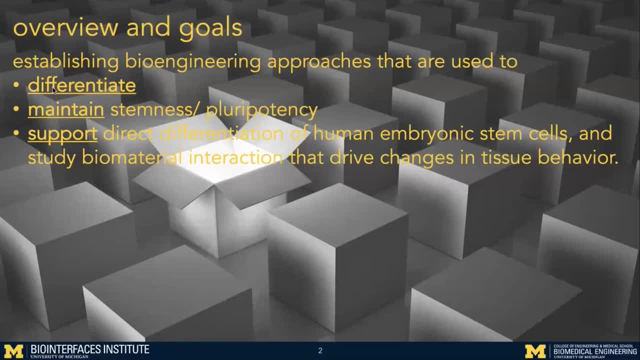 Okay, the overview and goal for this project- I mean not this project, these the projects that I'm going to talk about- is basically establishing bioengineering approaches that are used to differentiate, maintain and support human embryonic and pluripotent stem cells to study. 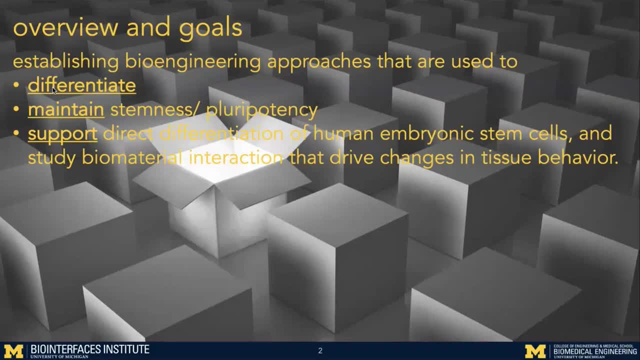 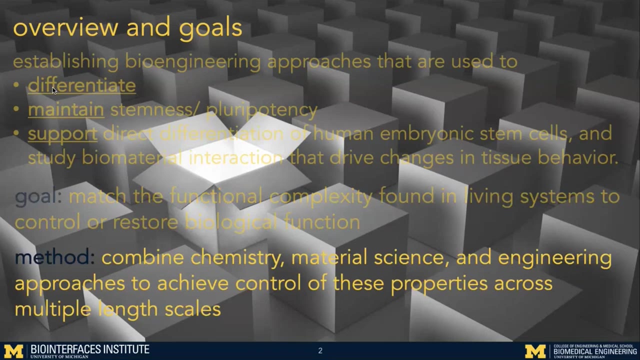 biomaterial interaction that drive changes in tissue behavior. To do that, our goal to match the function and complexity found in living system, to control or restore biological function and or methodology- is to combine chemistry, material sciences, engineering approaches to achieve control of these properties and multiple length scales. So, as we all know, 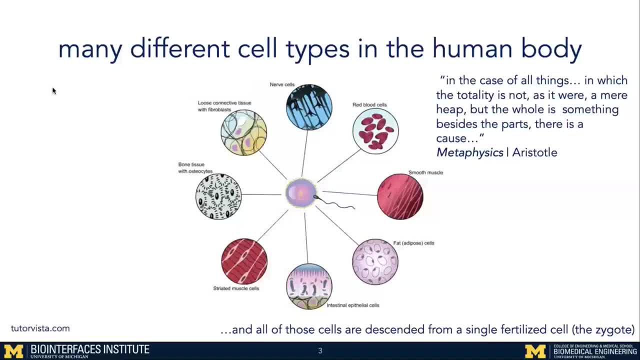 all the cells in the body. it's coming from one cell type called zygote, And it's it's called zygote. You can make them from red blood cells, nerve cells and tissue cells and and whatever you can think about it. so, um, this is a time lapse, um, from. 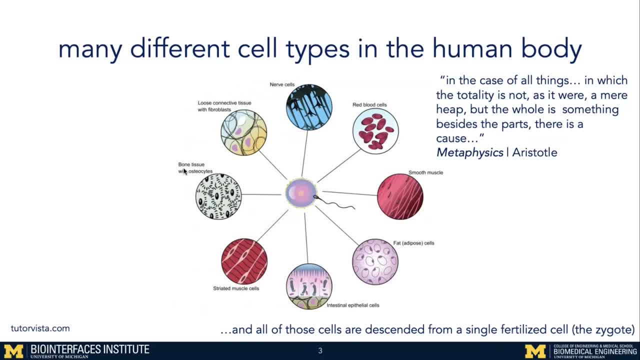 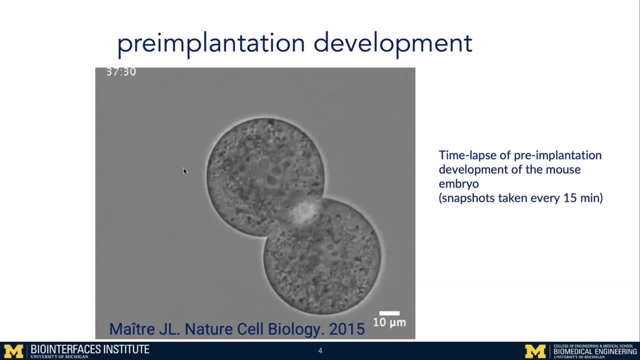 miles embryo. this in pre-implantation development, as you can see, one cell become two. therefore it increases two to n manner, like exponentially, and at some point- and it started, it's like the embryo, the um, the egg starts hatching and it's going to the uterus. but we're going to talk about most of. 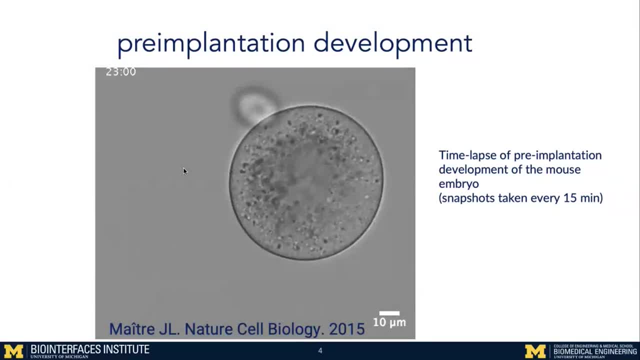 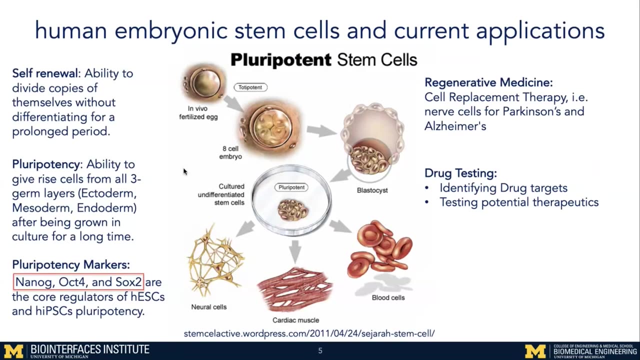 the part of it at the first part of the talk about, like, early development, and later on i'm going to talk about different methodologies. so, to brief, i just wanted to um draw your attention to human embryonic stem cells, or pluripotent stem cells. we know that they're, they, um, they um. 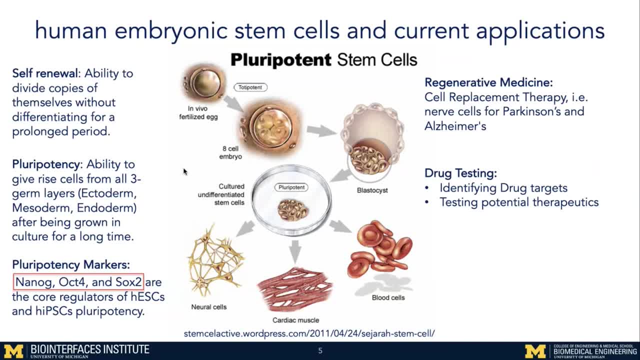 they have ability to self-know and maintain. pluripotency, meaning suffering, means like they can make their copies of themselves without differentiating for a prolonged period. and pluripotency means they can make like three different germ layers: ectoderm, mesoderm. endoderm means like you can make like neuron cells or bone cells and and whatnot. 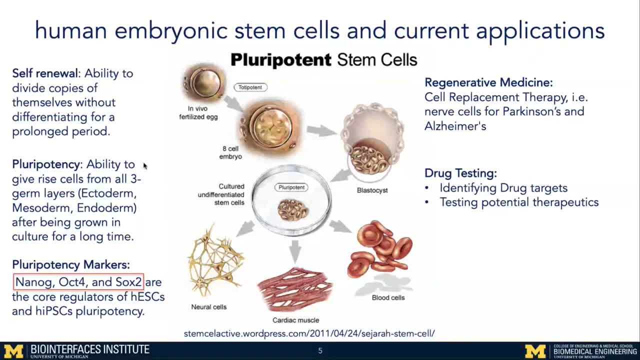 so i just want you to pay attention to these pluripotency markers, because i'm going to talk about this three most of the time in my talk. um, none of awkward and sucks too. these pluripotency markers are the core regulators of um to maintain pluripotency of eecs and ipcs. if you see any of 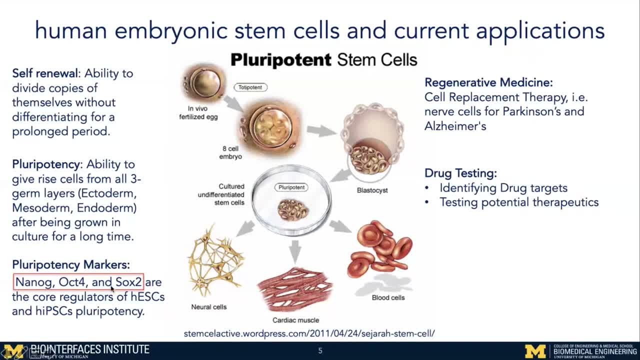 those links in the description below, i'm going to show you some of the markers that i'm going to show you. so if you see any of those links in the description below, i'm going to show you some of the. from the nicholas. it means that these cells are differentiating three of them. i mean, if three of 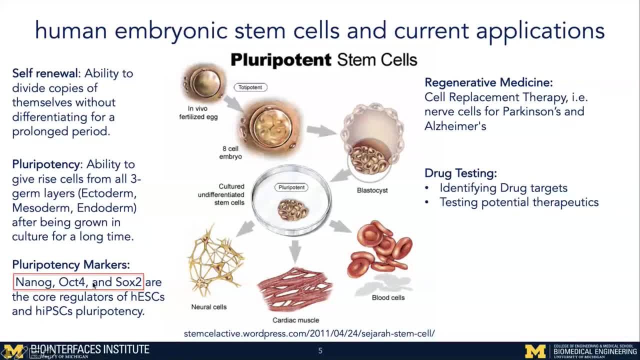 them um, maintain, um, if they are three of them is just like localized in the nicholas, they, i mean they are undifferentiated. so so what are these cells? what are we going to do with them? so we can use the cells for in? to use in regenerative medicine means you can use them for cell 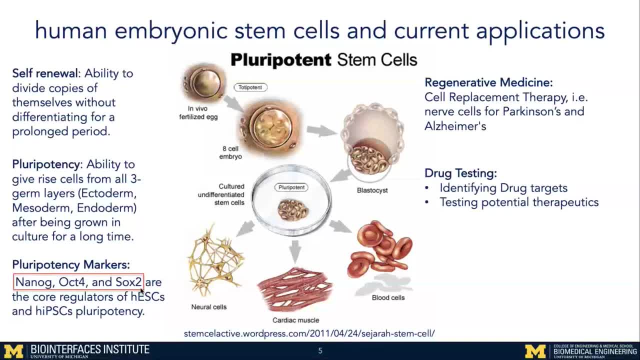 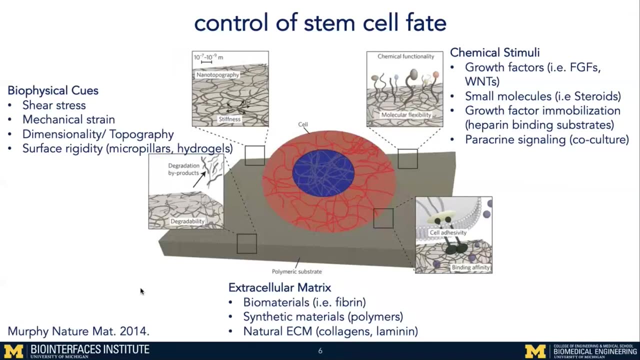 replacement therapy, like using for perkinsons and alzheimer's, or we can use these for drug testing, like identifying drug targets or testing potential therapeutics. so, researchers, so far they've been using different strategies like, for example, biophysical cues, excess telemetrics or chemical stimuli. basically, they're like a lot of like approaches to control. 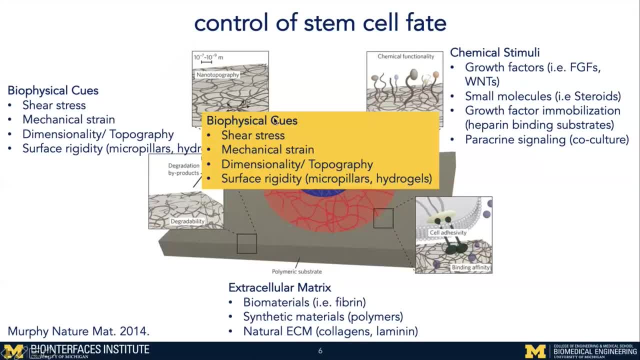 it. so in the first part i will be talking about talking about biophysical cues, main mainly mechanical strain, applying forces to the eecs to differentiate them. so sorry, um, and researchers in the field, especially in the field of biophysical cues, are going to be using different strategies. 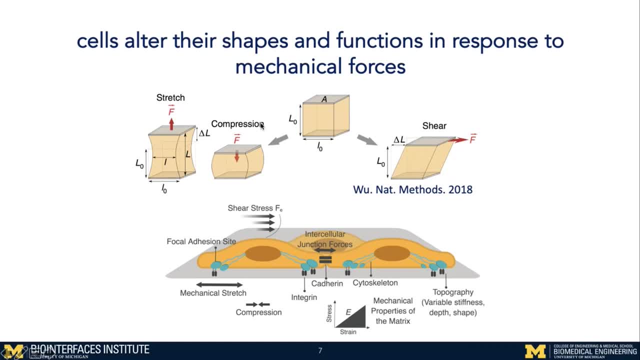 to understand how these forces altering um cell fate or understanding the um, but understanding forces in the body. in this case we know that there's like stretching in the body or compression. you can think your teeth or you can think like sheer stress in the in your blood vessels, because 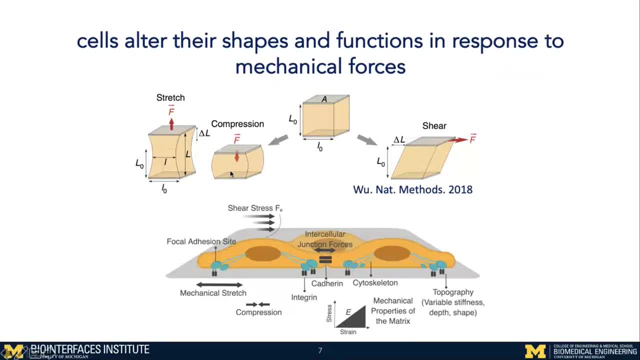 they become more most likely like a flat-ish um shape. due to all these forces, the cells they change their um. there's a term called tensegrity and it's a term that's used to describe the tensegrity or mechanical um, mechanical biology, part of it, by um donald inger, so he basically um. 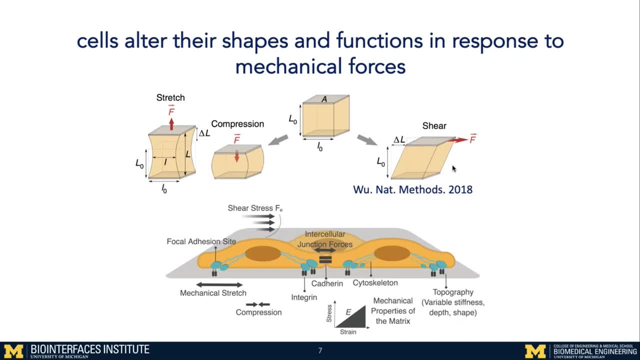 introduced this term back in the day, saying that due to these like forces applying to cells, the um, the tensegrity of this like cell that it's changing the force, changes the cell behavior. in this case, you apply force. in this case, like, for example, mechanical stretch, you apply this. 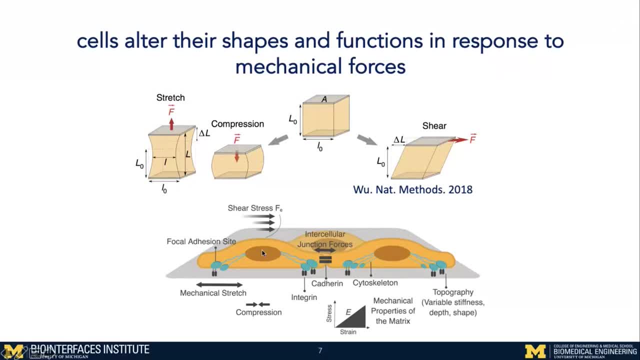 force to the intake- inner greens are getting it. and then focal adhesion, kinase activating, and then cytoskeleton and changing nichols, gene expression protection, blah blah blah. so this is just like over, uh, overview. so there are like forces in the field. um, especially engineers have been 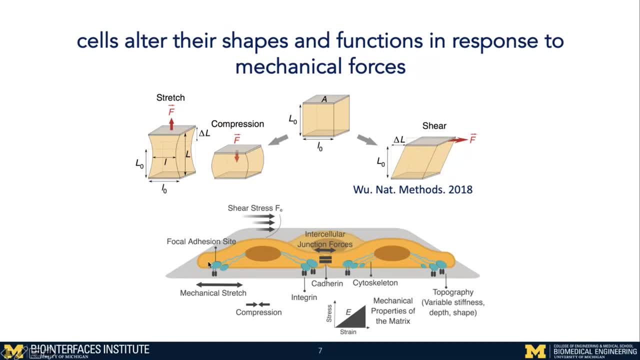 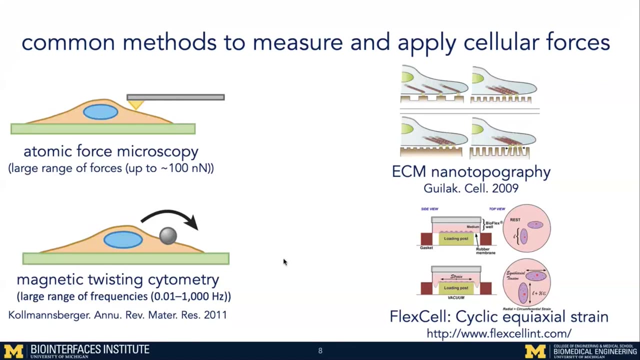 using. there's one called atomic microscopy. you can use this up to 100 nanonewton, or you can use magnetic tweezing cytometry. basically, you introduce a beat and you can um move, move this beat through the um tweezing cytometry. and there's also called uh nanotopography, ecm nanotopography. basically you 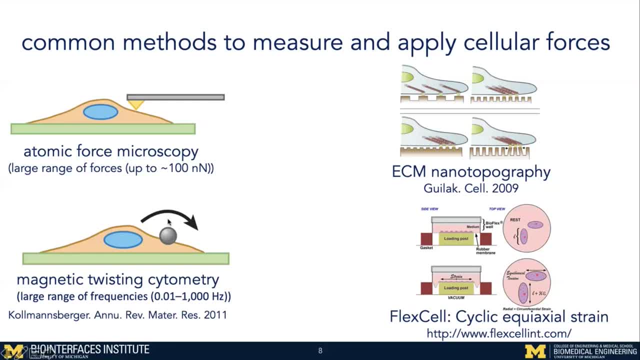 can use uh nanotopography to make this surface stiff or soft and understand how the cells are behaving. or you can use vacuum based um like, um the mechanical strain, um. this is a flax cell, it's a company that um you get, basically using vacuum and applying strain from two sides and basically 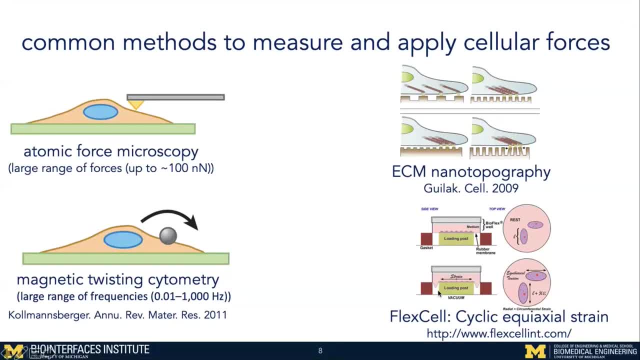 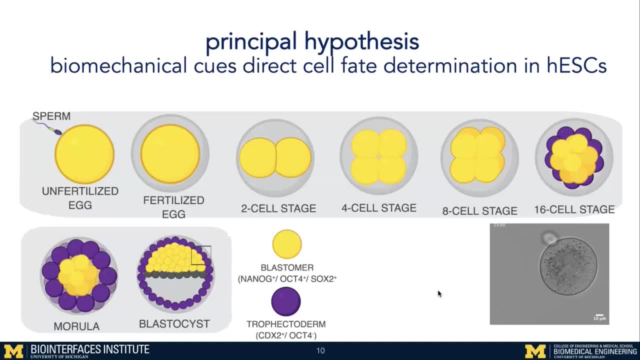 applying force to cells and understanding how they react. so how do physical forces alter stem cell fate during development? so the principal hypothesis coming from from, as i mentioned earlier, um fertilized cells become like two cell, then four, eight, sixteen again. it goes two to n manner exponentially, and at some point the there's no, there's no growth. 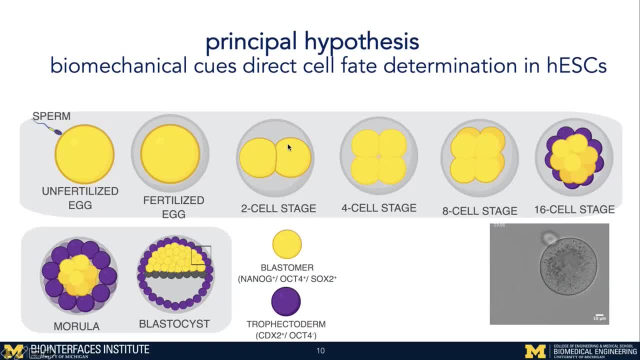 factors, or there's no, um, there's nothing in from, there's nothing coming from outside inside and nothing getting inside outside. basically, everything happens in the, in the egg and, like you can think, the egg, like you eat daily. so, um, when they reach the 16 cell, they start like they actually before. 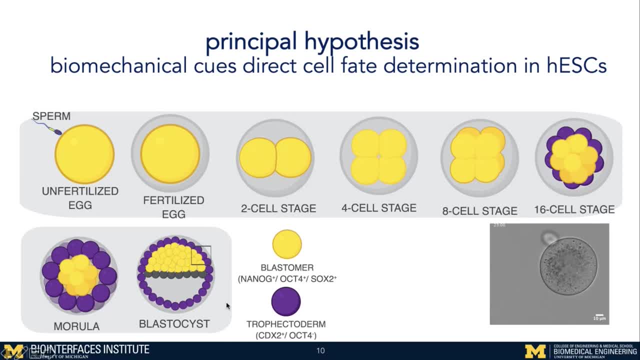 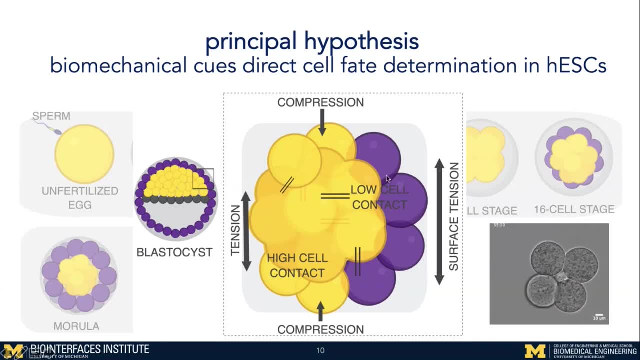 that it is. they start differentiating. and um, the principal hypothesis, um, when i was like working my phd, just like, oh, there must be a lot of compression forces or low cell contact and surface tension and compression forces. these are the portions of starting these cells to 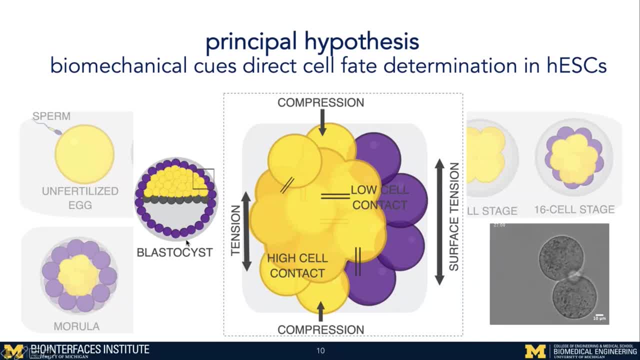 differentiate because, before hatching these cells, they know what to become next. like, for example, um, purple, the color, um, i put it as like a purple, these are making, gonna, uh, these are gonna make the placenta, how do they know? or these like, um, these like, and then these, uh, the gray and the. 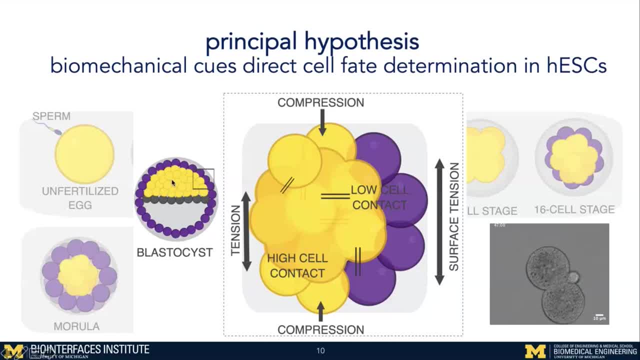 yellow. they, like the escs, are coming from the like, very temporary from this side, and there's, like the um, early, early endoderm layer in this area. but how do they know how? what to become next? so, to just to test this hypothesis, we wanted to: um assess the effect of integromediated 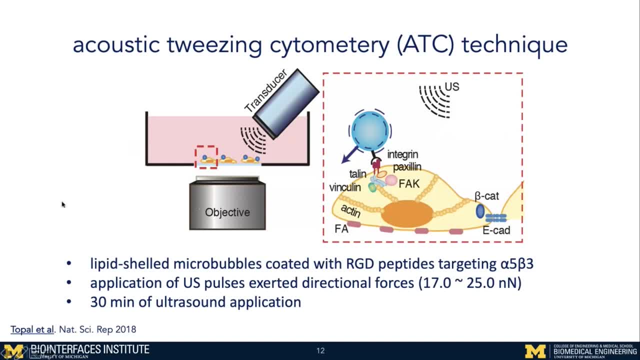 cyclic um cyclic strain on escs and to do that we um established a protocol or a technique. i mean i i will be referring as atc acoustic to wheezing cytometry. basically, we use um ellipid shelled micro bubbles coated with rgd peptide targeting alpha b, beta 3, and apply 45 degree angle with 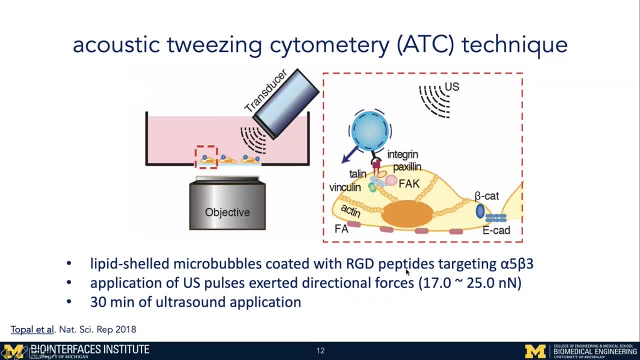 apply ultrasound to the cell for 17 to 25 nanometer and we apply for um 30 minutes ultrasound application. as you can see, this is basically the technique that i will be talking about the first part of the talk. so, as you can see, here we first applied these forces to single. 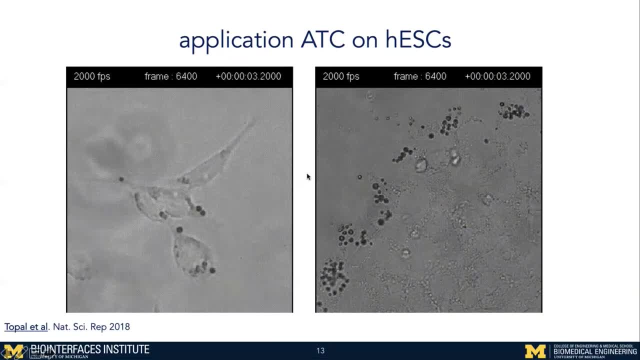 cell level, on colony level, and we wanted to see how they react, as you can see these black dots there, or micro bubbles, and it gives. you can see here too, it's in the colony, uh edge of the colony, and when we apply, let me give these bubbles um, to these um cells, they prefer sticking on the periphery. 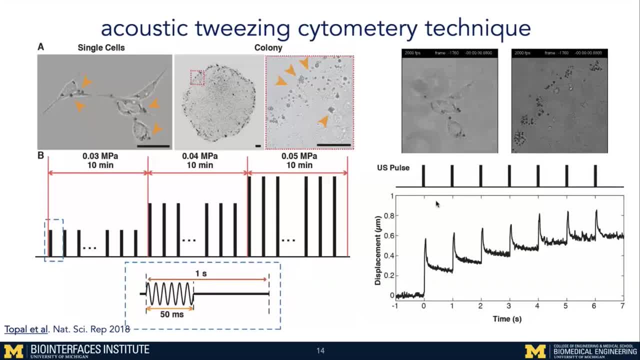 of the colony, not in the middle. so the next we um. i just want you to pay attention that how we do it is just like- again, this is like single cell colony and um. we apply for 50 milliseconds and 10 milliseconds of duration and we apply for one second for that and then we do it just like for. 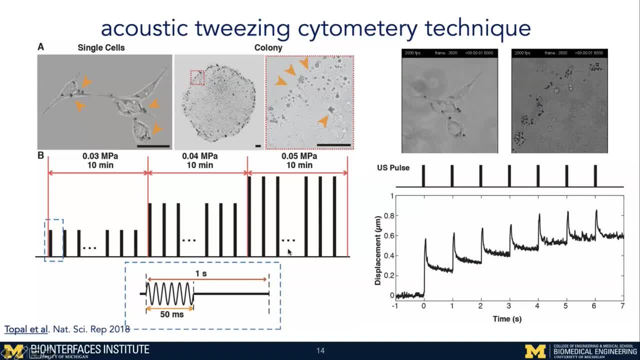 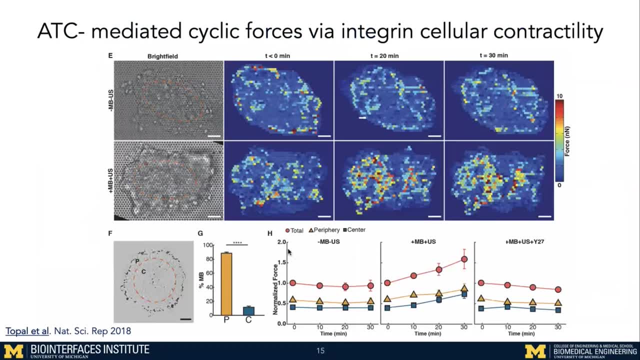 um 30 minutes, and we apply force, stop it, apply again, stop it, so vice versa, all right. um, these are just like the only two uh steps that we know right now, and we have to apply for the second and we have to apply for the third step for that. so, okay, let me just pause this for a moment. 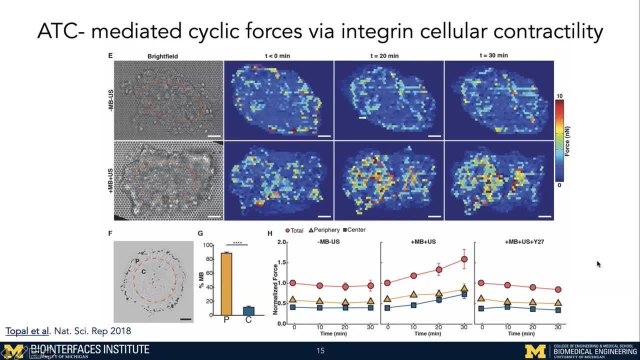 i can see. i can see, u know, i can hear you can you can still see me? i'm not sure, because there was a thing here. it's disappeared. hello, you apply ultrasound forces, how it's going to happen, the contractility. so for this um experiment, we use micro pillars, as you can see here. the pillars, so we apply. we did this with the jumping. 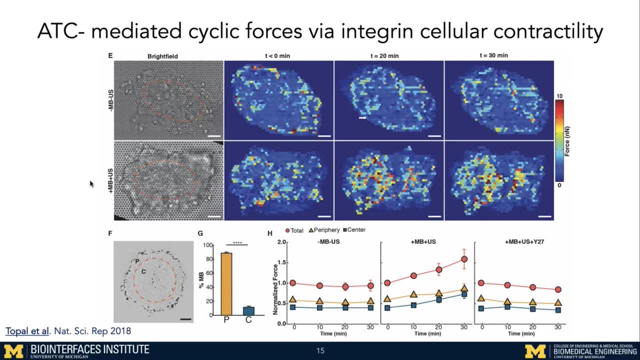 for this group at the university of michigan mechanical engineering, um, we put the um with the micro pillars, we put the cells on it and then this is like no bubble, no ultrasound. and this is bubble and ultrasound. at the beginning you don't see. the red color means there are a lot of 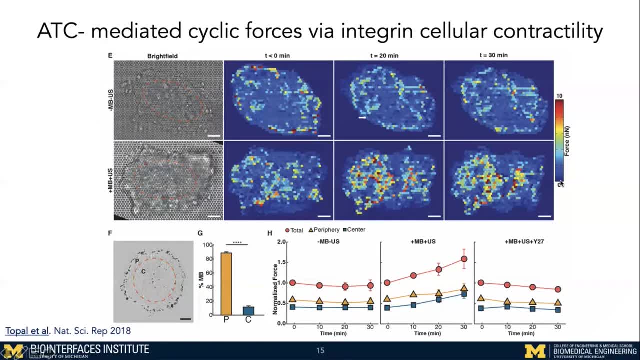 contractility. blue, it means there's nothing. um, as you can see here, at the beginning there's nothing and then like nothing, not nothing, nothing, it's just like, not like perfectly blue. but i want you to pay attention here: after 30 minutes we apply forces and, like i mentioned earlier, the bubbles. 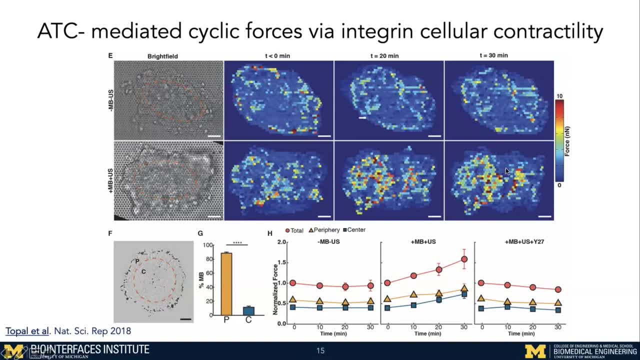 are like, located at the periphery, but when you apply forces, the, the contractility accumulate in the center of the colony and we tested this with the normalized force and we applied um, an inhibitor 27- it's basically a rock inhibitor um- and we tested this: whether, if you apply the rock inhibitor, 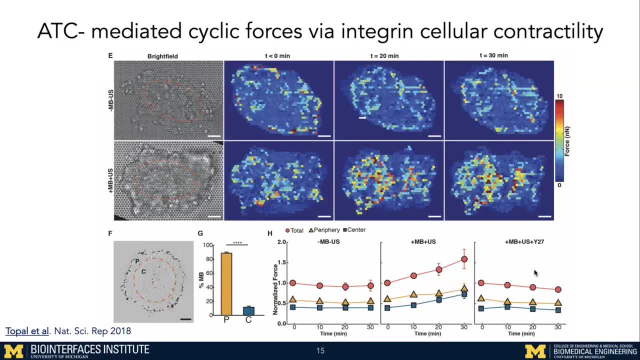 whether contractility is a habit or not. and then, when you apply the fly to inhibitor, we were not able to get the contractility as um, as without the um, what is it the inhibitor? all right. so since we work with the ecs, the next question is just like: okay, this is human embryonic stem cells or full. 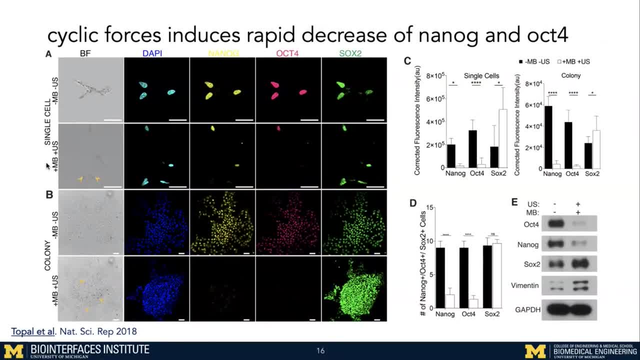 upon stem cells. have you checked in on our foreign sucks too? and yes, we did. and, as you can see here, the single cell level and the colony level- at the single cell level you can see not gonna afford disappeared and sucks to expression is still there. and we did the same thing for the colony level, applying 30 minutes of forces and 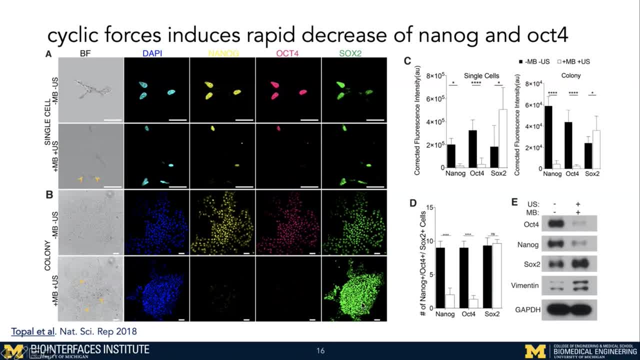 not gonna pour disappeared. sucks to expression is high and we- this is like- only the confocal analysis, the image technique, and then we wanted to correlate with the protein expression analysis and we did the awkward sucks to nanoc, again with and without micro bubble and ultrasound, and as you can see here there's like after 30 minutes of for non-normal. 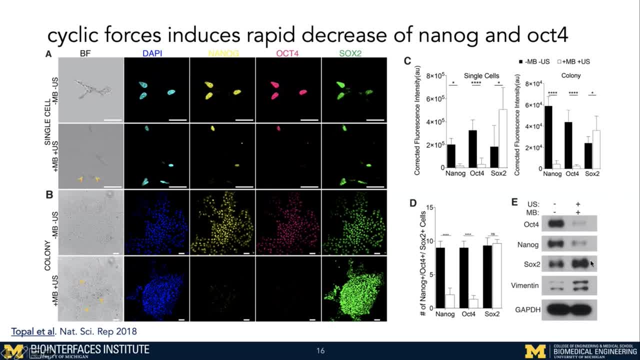 expression and then the cell level disappears and sucks to um over expressed. and we were just testing and fishing multiple um antibodies and we wanted to see whether um, since this is like a real differentiation- whether we can do the emt. uh, we wanted to test momentum and then we've seen. 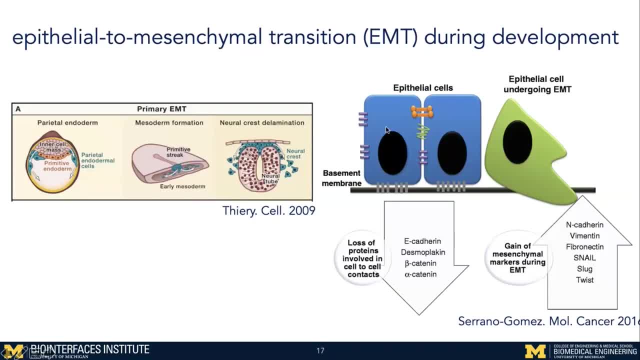 momentum expression is high means these cells are going to epithelial, to mesenchymal transition and this is very well known in the field um uh biologists- they were able to figure that out like they're going to primary emt and um they, before they make a neural crest elimination, they start. 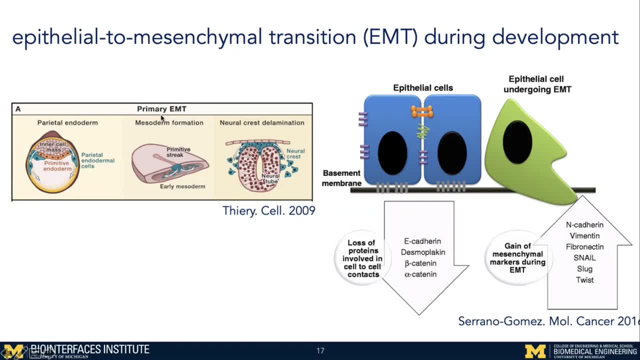 they, they are going through epithelial mesenchymal transition. so it's also another um paper about talking about if the e-cad here in beta content and alpha content, blah, blah. they go down, means these cells, um, and the momentum and coherent program acting goes up. it means that the cells. 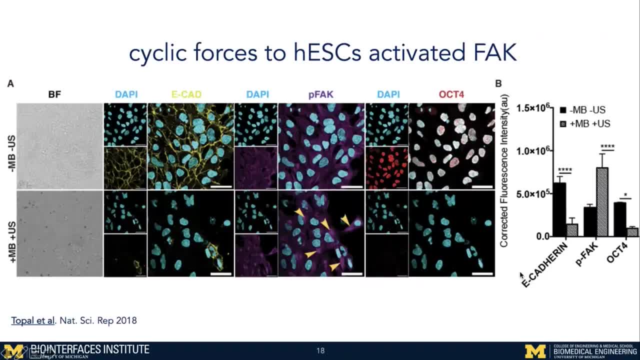 are going to emt transition, so we tested this before that. i want you to show that, like um activation of focal adhesion kinase. this is very important in the field of the human embryonic stem cells because, um my, um my colleague, he was able to use this activation of focal adhesion kinase. we used a manganese treatment for. 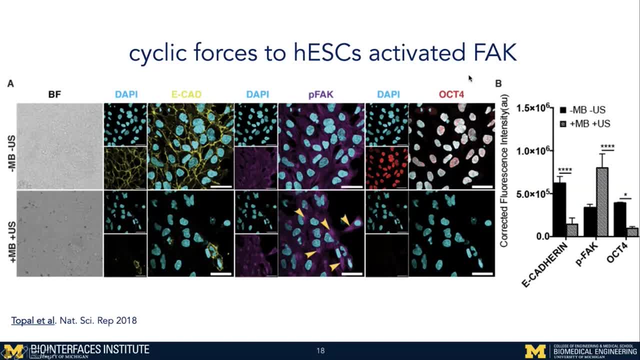 48 hours and he was able to see activation of fact and basically um, um, basically triggering human embryonic stem cell to differentiate. so we tested the same hypotheses with ultrasound technique, the atc, and we were able to get phosphorylation of back um localized in the 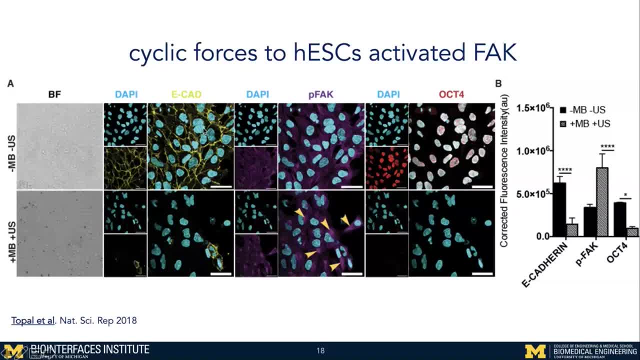 one part of the cell and at the same time, since we were, since we were able to see the momentum increase and we were like, okay, what's going to happen with e-cad union and n-cad hearing? and yes, um, e-cad hearing is highly expressed in human embryonic stem cells and when you apply the forces e-cad, 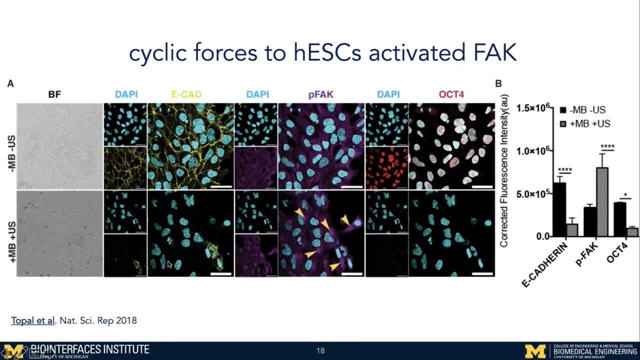 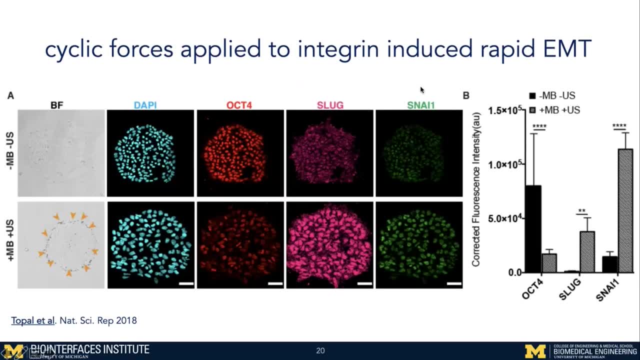 hearing is lost. so these cells are definitely going to epithelial, to mesenchymal transition and be further tested. but it is true- and yes, we did the same big word in cat hearing- and be further correlated with slug and snail because those are the um markers of rapid mt induction. so the next thing is: like biologists they were able to figure. 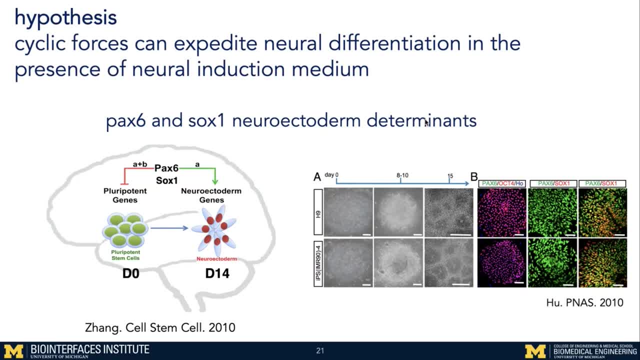 that out. um, how, pacs, um, how to make neural rosettes and neural differentiation. they were on 2d. they were able to do pac, giant sridhar, one is at early neural exothermic determinants. um, they were able to get this from at date day 14. they named them as a rosette, or we can call them roses. against these older brains- um, that's what they named them, not rosette, or you can call them roses- movements of life, especially in the frontal lobes. certainly Celebrina can proprietally das, then we mmta. we want to see this umARS lab too in Illinois, and we will be able to get a clearer life and 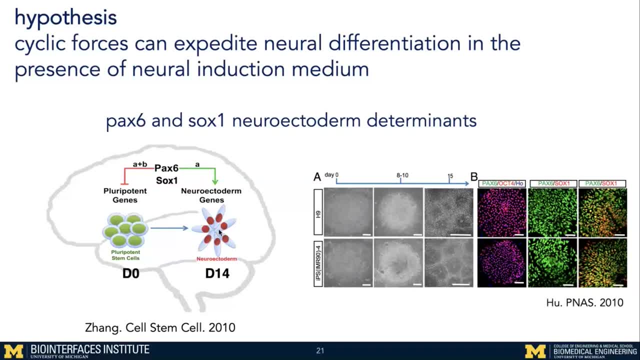 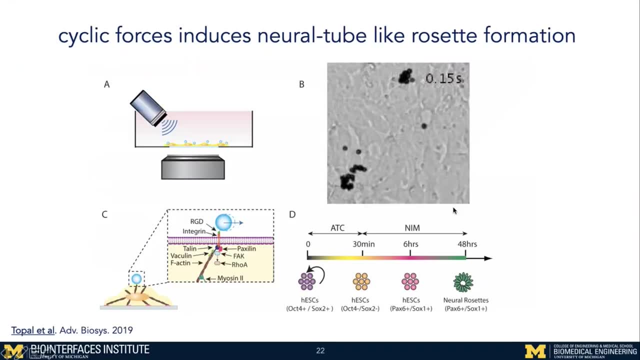 work in mine too. so if you're thinking about doing such experiments, could you take our next? oops, see it. but they are so smart they were able to figure this out, like at day 15, and they called them um, and then we wanted to test this hypothesis with our technique. better we can um decrease that. 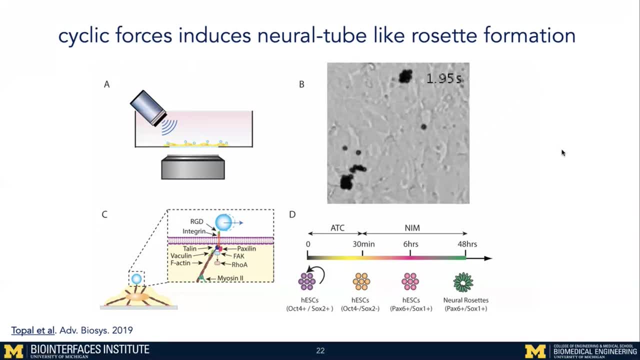 time point means they were able to do for 14 days, two weeks, basically whether we can just put it down and whether we can really mimic early embryo on 2d though um. so we did exact same technique: we apply the force and then after 30 minutes we gave them neural induction, media um, and then and then 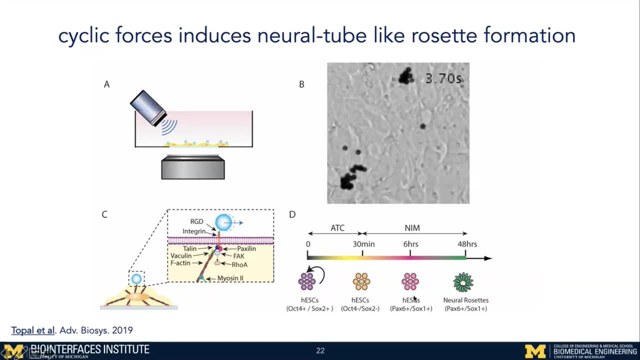 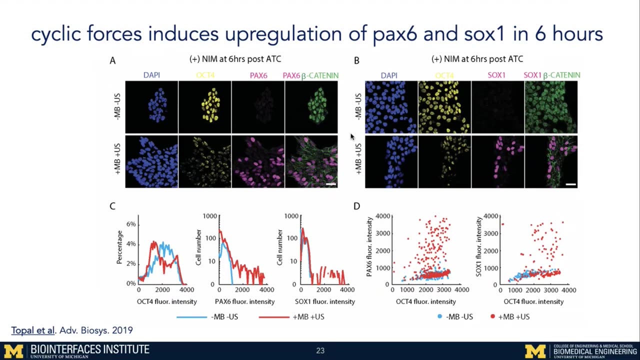 we continued for up to 48 hours. at six hours we started seeing pac-6 and sax-1 expression and 48 hours we started seeing pac-6 and sax-1 expression and rosettes. so as you can see here, this is early um determinant of upper relation of pac-6 and sax-1 in six hours and later on, bam here. so we 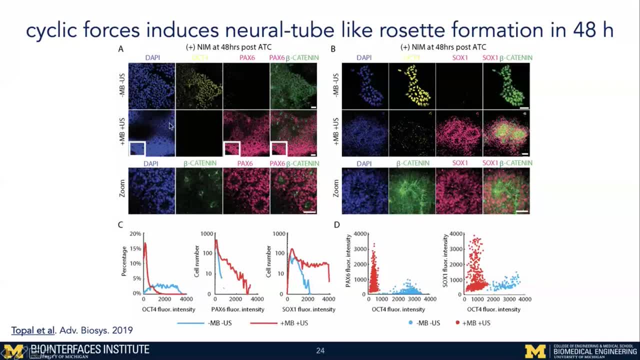 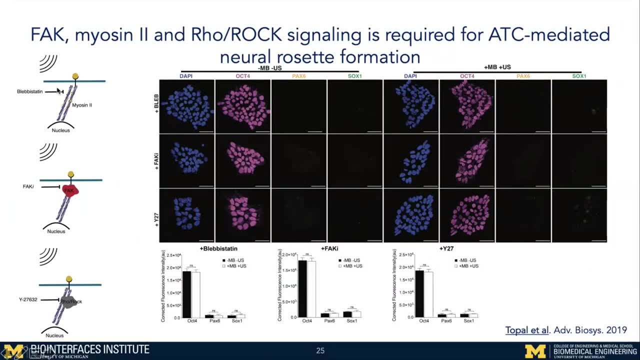 get the rosettes, um, after 48 hours. so and then we wanted to test our hypotheses again with the inhibitors. so we did like: uh, what if we block myosin 2 with the blob of statin or focal adhesion kinase inhibitor? and again, 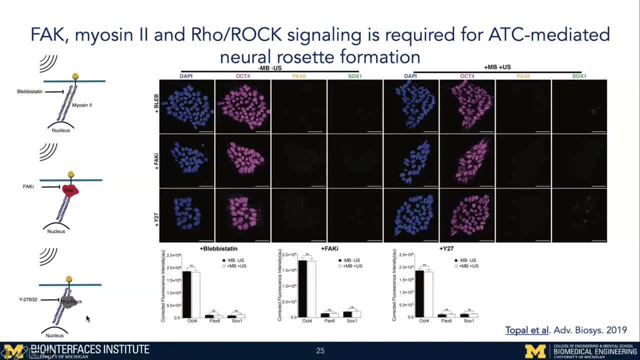 rock inhibitor and, as you can see here, we did not get any of those markers upregulated um once. we gave them um the inhibitor because they basically inhibit the pathway. so our conclusion of the from the first part is like: basically, cyclophore should generate rapid mechanotron responses and eac's and it. 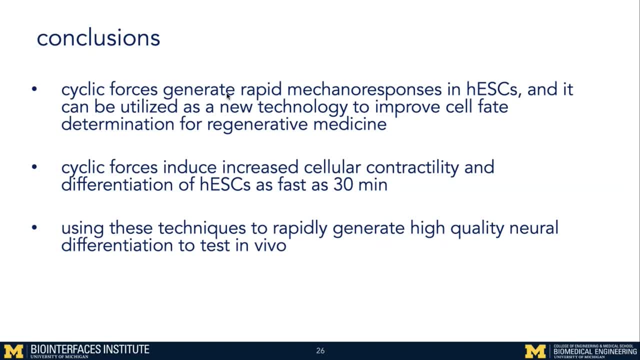 can be utilized as a new technology to improve cell fate determination and for regenerative medicine. and cyclic forces into the induce increased cellular contractility and differentiation of eac's as fast as 30 minutes, using these techniques to rapidly generate high quality neural differentiation to test and evo. so the next part. i will talk about the excess matrix part of the 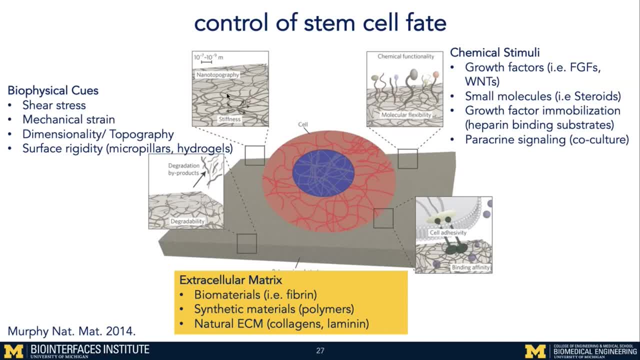 controlling stem cell fate: basic review. i will be talking about um synthetic materials, that how we can alter stem cell fate on it. so to do that, um, um, let me just give you a little bit of an example. let me just give you a little bit of an example. um, let me just give you a little bit of an example. 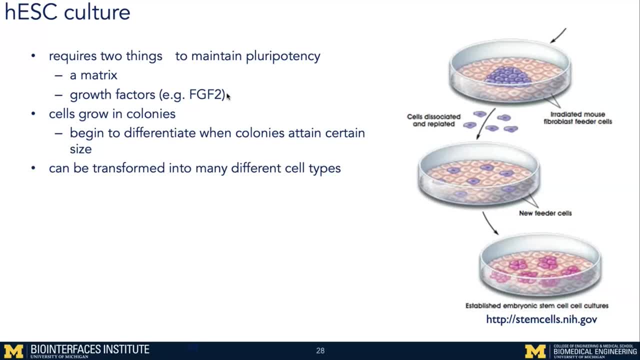 um, let me just give you a little bit of an example. um, let me just give you a little bit of an example. like i mentioned earlier- eac- i did not talk about how to be cultured. i just talked about how um they react, how where they are coming from and whatnot. so um easy culture or poop on. 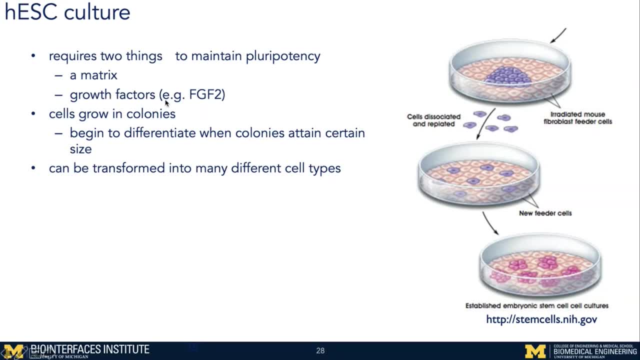 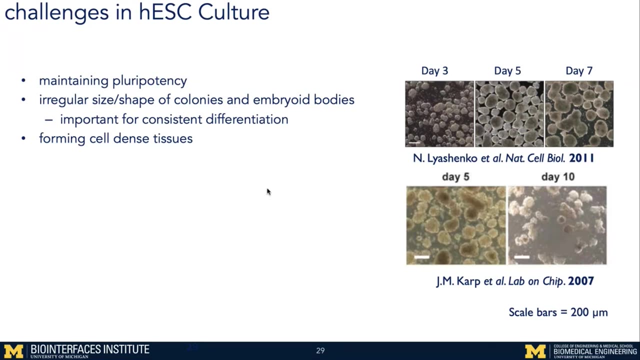 stem cells they need, um two things: a matrix and graph factors so cells can grow in colonies and they can transform to many cell types. so, um, there are challenges to maintain propensity and because, um, they have irregular shape, they make irregular- i mean also you make it in 3d- they make irregular shape in colonies and rebodies and they form cell dense tissues and 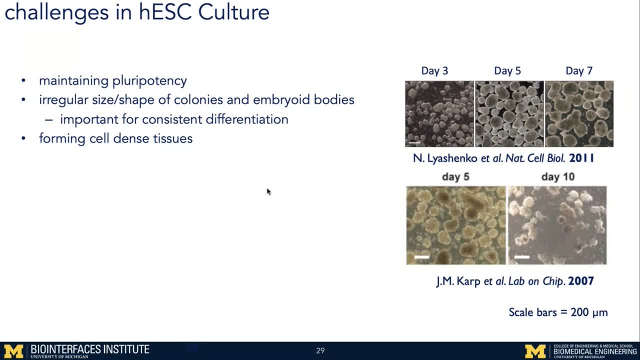 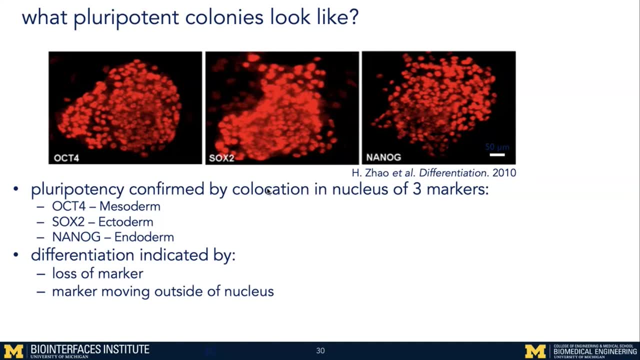 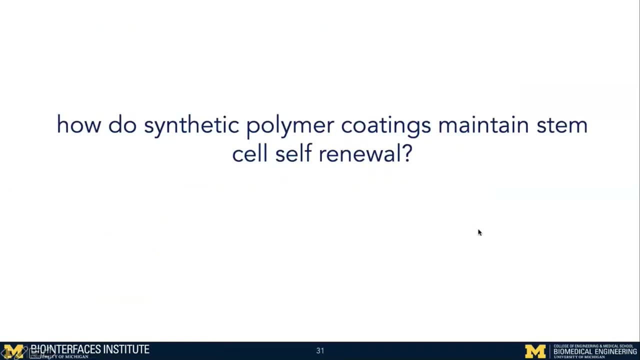 they start differentiating spontaneously. so this is how they look, how eac is looking like as a, like a clamp or colony, um, and like i mentioned earlier, if you see them in the necklace there, it means they are undifferentiated, can grow in colonies and they can transform to. 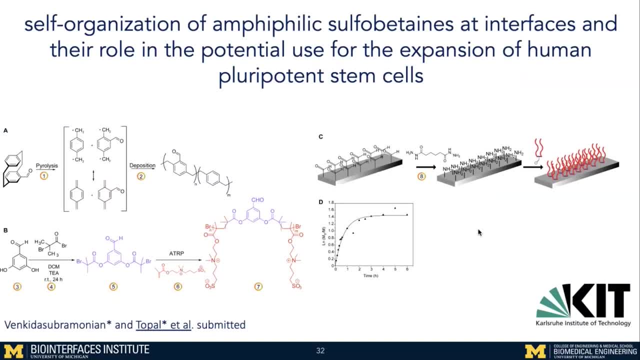 many cell types using stem cell for noah. this is the study that we did um at the german group, i mean germany carlton institute of technology. basically, it's a polymer, uh, zwitterionic, it has plus and minus ends, um, uh, we, we use this polymer because um before me in my lab and your glans lab, they 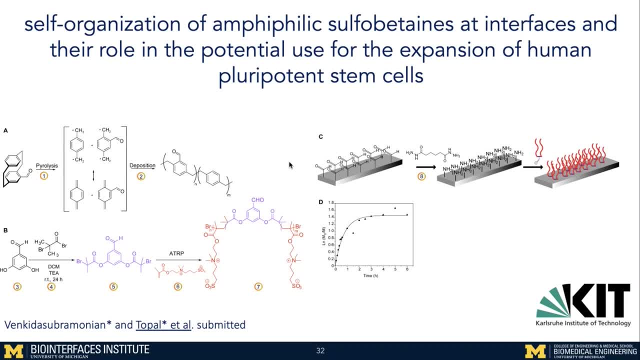 were able to um figure out and they published that in nature biotech paper about epimax polymer that i um the polymer that supports engineering stem cells um cefrenuel. so we did, we altered a little this polymer and we uh investigated the same way whether these we can um maintain pluripotency on. 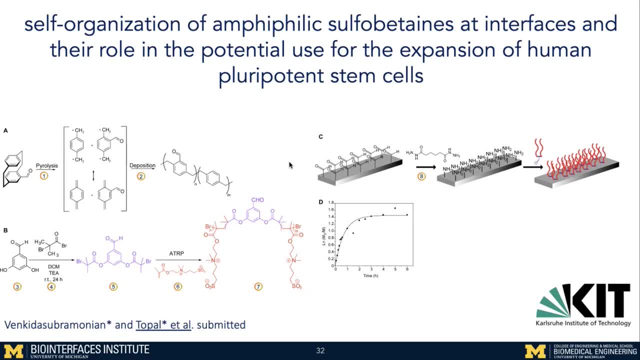 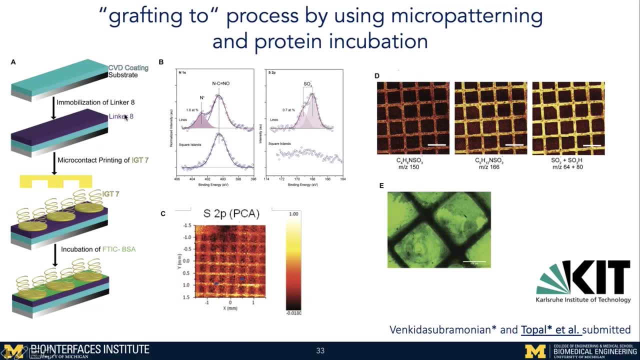 this polymer and yeah, so this is the german part of uh part of it, how they did it, using the cbd coating substrate and using the linker, using micro contact printing and whatnot, and later on um gotham, he did this work, part of it um he she was able to use the um protein. whether we can um. 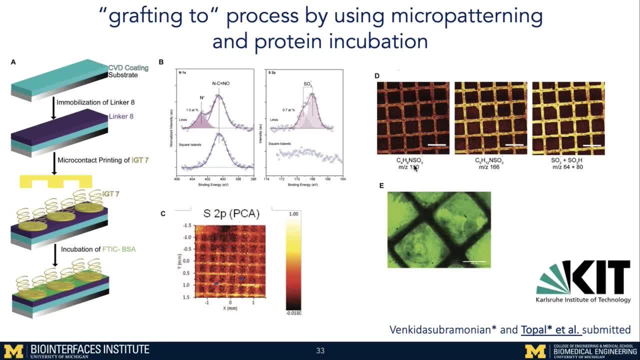 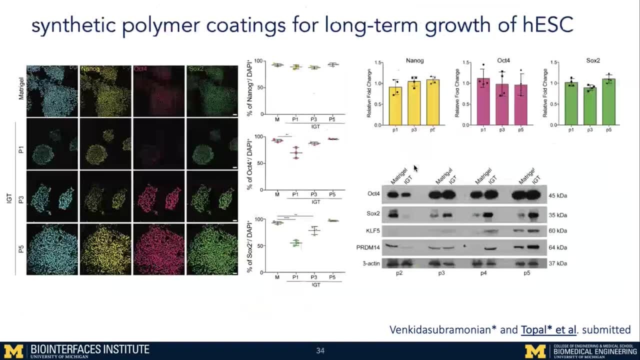 emit, put the protein and whether they're gonna absorb the polymer or not. so and then the next thing we want, since um, we wanted to test whether we can maintain um stem cells on it and or control group, of course, metrogel, because this is like um. everybody used the metrogel um at the at the 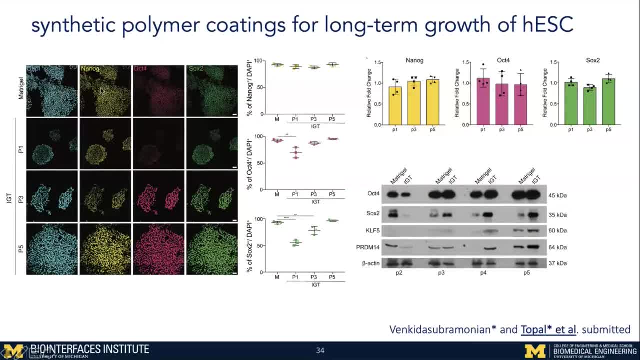 beginning of the passage one we get like teeny, teeny colonies and later they get used to it. at passage five and we correlated they were able to maintain proponsive, that differentiating, and we did the western blood analyses, as you can see here. um, the beta actin is a control group and 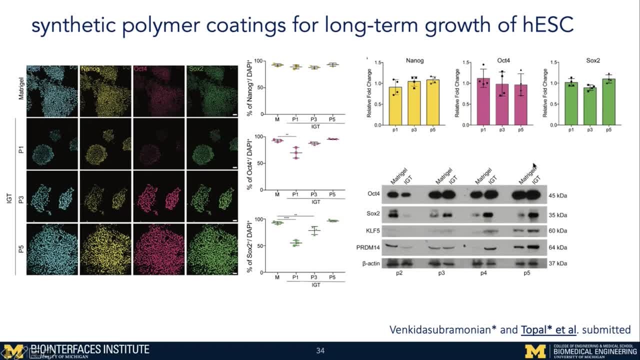 these are the pluripotency markers. this is a new marker, um, after five passages and, as you can see, they're still like highly maintained their propensity. and this is qpcr analysis. it means there's no um, there's no changes in the gene expression. so our conclusion from this part of 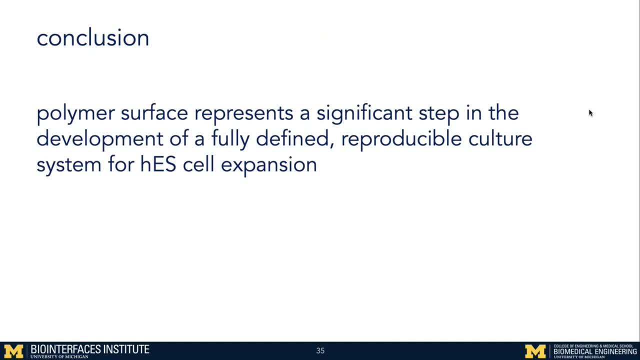 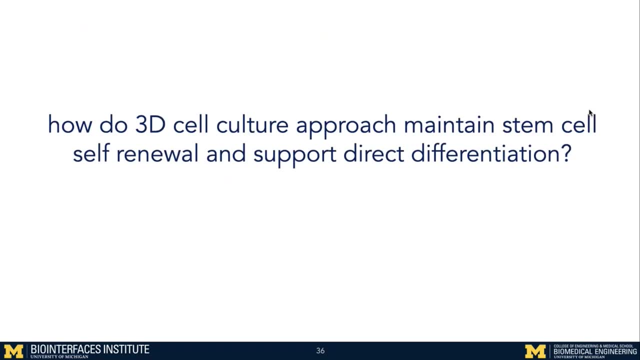 the work is using polymer surface represent a significant step in the development of fully defined reproducible culture system for ease for cell expansion. so the next part is: how do a 3d cell culture approach maintain stem cells? acronym support, direct depreciation. so basically using those three approaches in one. so we all 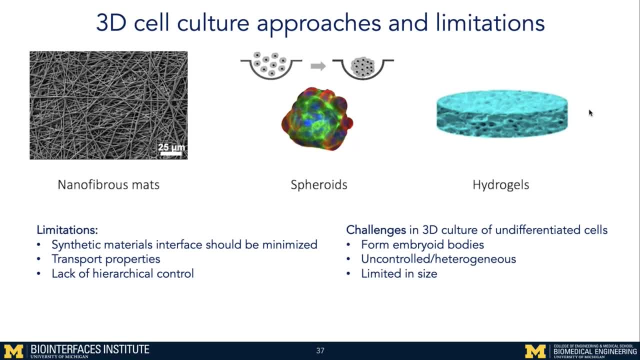 know the 3d cell culture approaches and there are like limitations. basically using um a lot of synthetic materials, it's not, especially if you're using for regenerative medicine purposes. it's no good. so we should- we should- minimize the inter interface for these materials. and also, uh, there are problems about limitations about transport properties and lack of hierarchy. 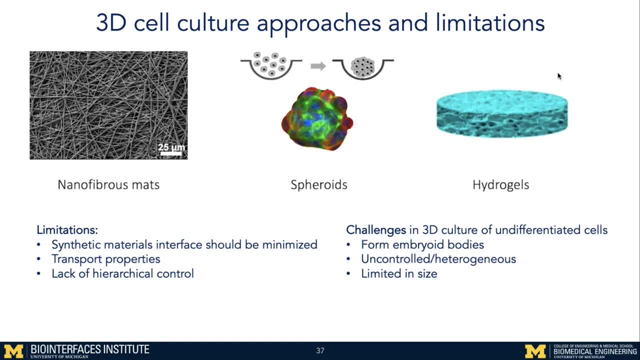 control and because, like you, you make it but you cannot. you cannot control the, the way it is, and other challenges like they, like 3d culture of undifferentiated stem cells. they are like forming embryo bodies, uncontrolled or heterogeneous or limited in size, and researchers have been using 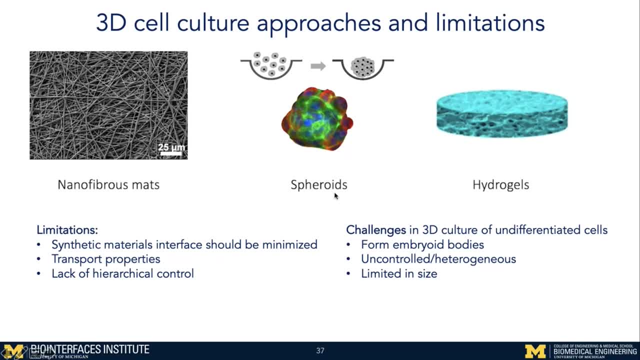 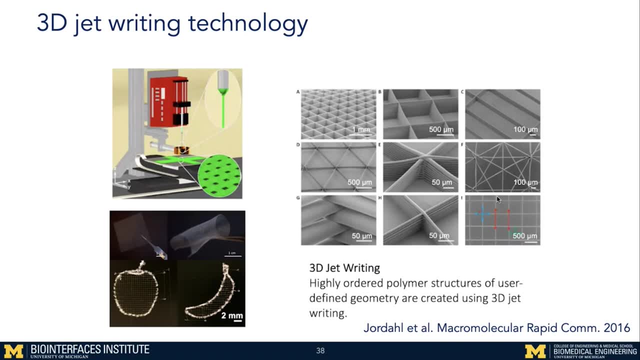 non-fragile mats, sprays or hydrogels to make 3d cell cultures. so in that case, um, this is jake's paper. he published this in 2016. um, it's basically a jet 3d jet writing technology. sorry, i said the um 3d jet writing technology. basically, you can. 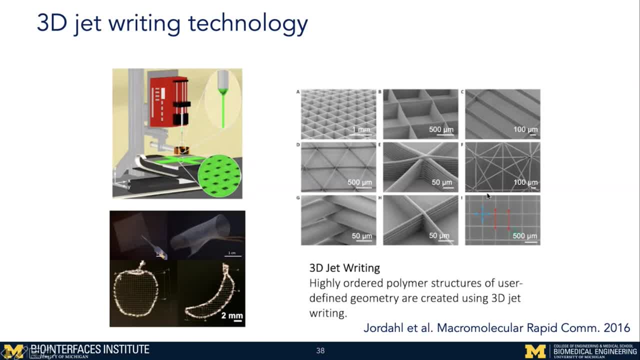 make like squares, rectangles or orthogonal, whatever you want. it's like, um, it's basically a scaffold, um you can. you can preach the size of the color, i mean not the color- um the, the size of the shape, whatever you want with this 3d printing. so first, in his, in his part, he wanted to test this. 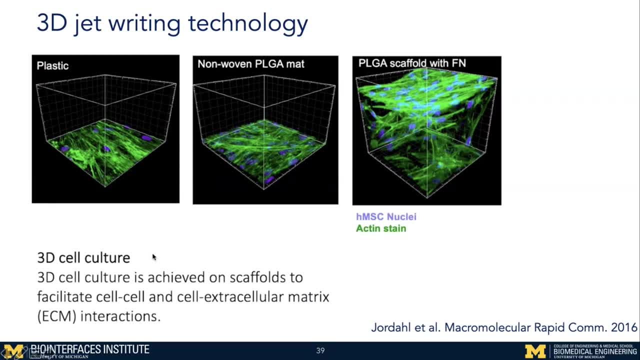 with the using um, um, this uh, this material, using um mesenchymal stem cells, and comparing with the plastic that 2d and novel and plga made on uh, on material too. and then he, he did this with uh just to show whether we can code with fibrinic as x-axis metrics and whether we can culture mesenchymal stem. 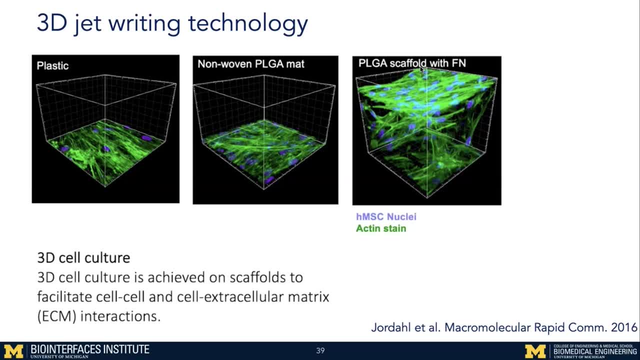 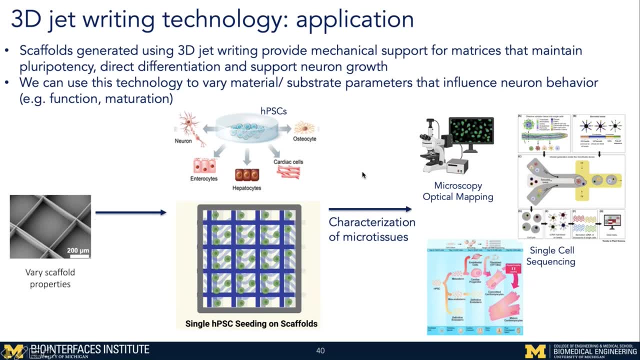 cells on an energy wasn't able to do it. so here we use this technology, um just for um, to provide mechanical support for matrices that maintain pluripotency, directing differentiation and supporting neural growth. we can also use this technology to vary material subservient parameters that influence neural 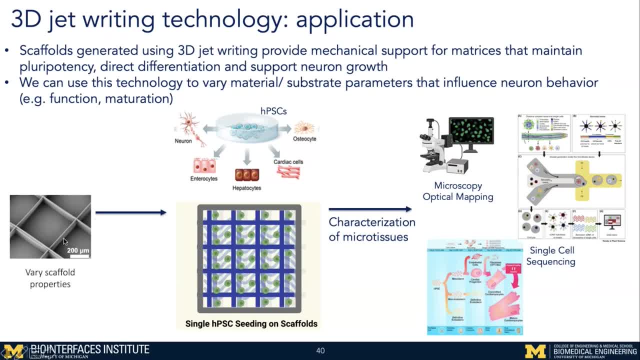 behavior. so how we do it, this is the part of the printing, part of it and then later we um, we do the existential matrix coding and then we see the human pluripotence stem cells on these, like i mentioned earlier, these pluripotence stem cells, they can make any kind of cells in this part of 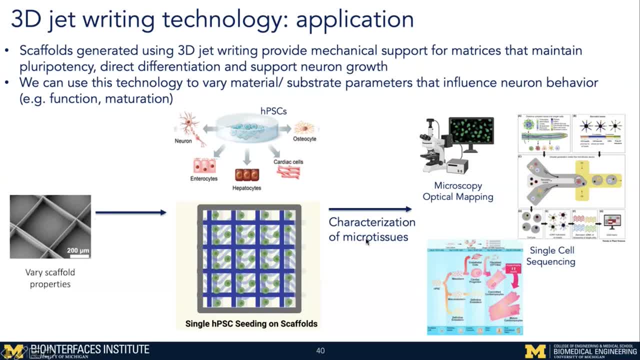 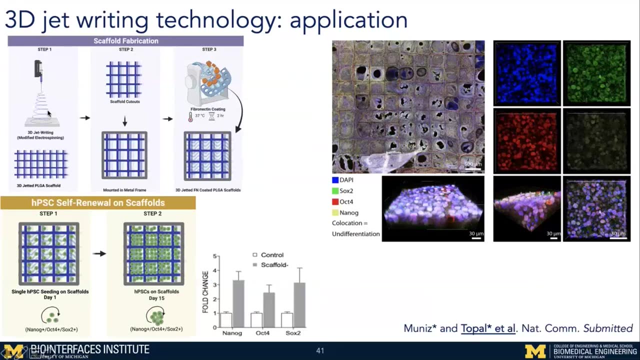 the um. in this part of the project that i'm going to talk about, we mainly focus on the neural part of it. so, characterization, we the um, i will be showing the images and the single cell sequence and not really, in this case, um. all right, so how we do it? so we do the 3d jet, writing as you can. 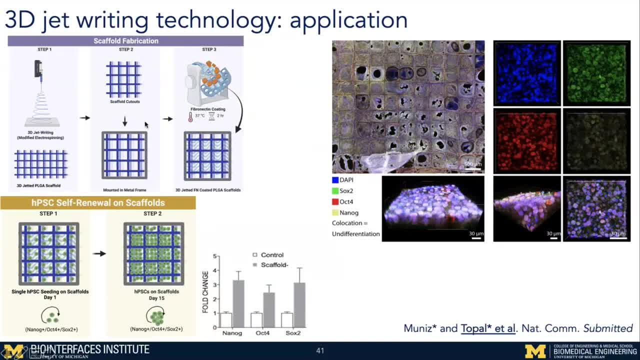 see here- and then cut them into little pieces and put them in a metal frame and doing the fibronectin coating for two hours, because these cells, yeah, they cannot just sit on a plga, so they need some cushion to sit on it. and then we give them like pluripotence stem cells and then at day 15 they maintain pluripotency. 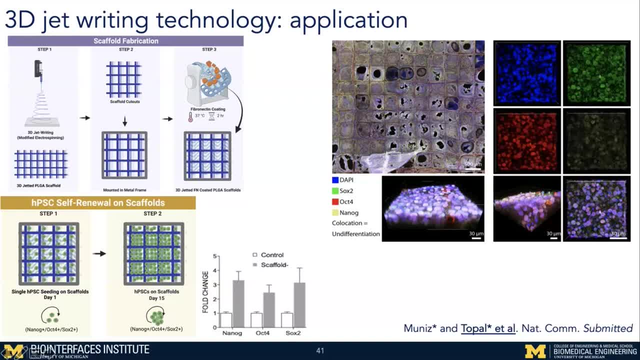 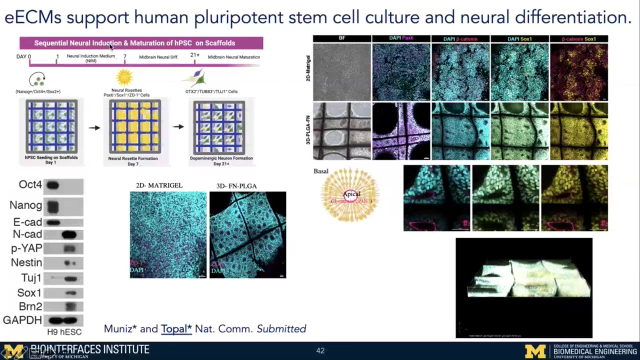 and whatnot. so here the data. so after 15 days you can see they've completely fully covered um the entire scaffolding and we were able to maintain the pluripotency and the cell renewal on these. so, and the next is whether we can differentiate the cells, your neural induction and maturation media on these. so to do, 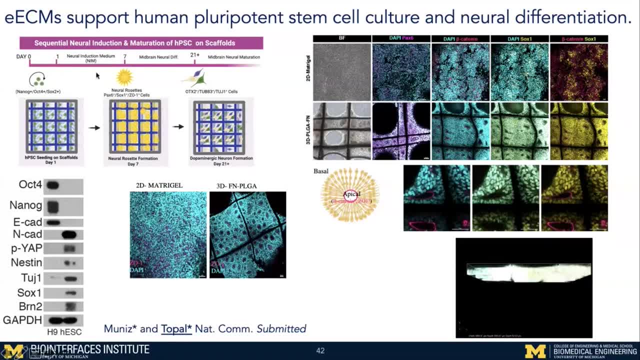 that again, at the beginning, we see the cells, we get a neural induction and you start seeing beautiful rosettes, like i showed you earlier in our um atc technique. and then after um, after 21 days, we get a neural at the beginning, mid-break differentiation. these are all um, um commercially available media, by the way, um so and then we give. 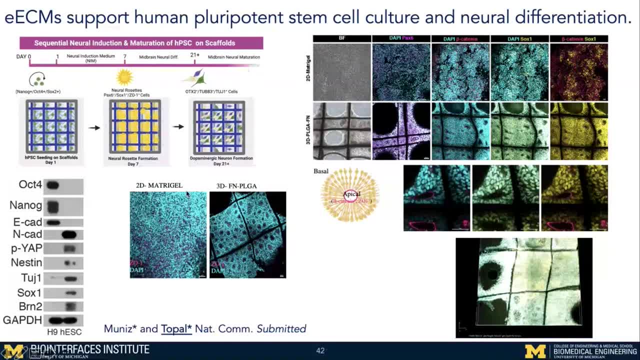 them mid-break neural maturation. so, as you can see here, they're like: uh, this is 2d, there's no um. after seven days there's no rosettes. but at the seven days we get the neural rosettes and later on i will be showing this is the three images of it and this is the western blood. 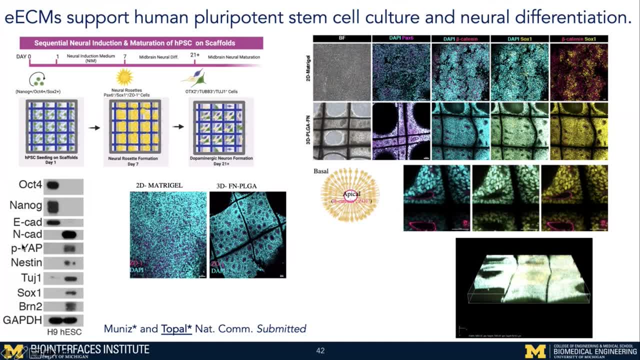 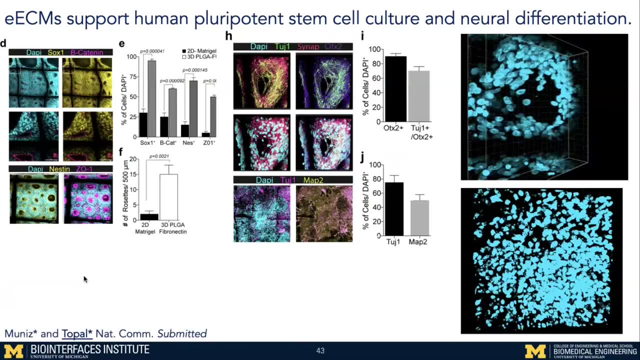 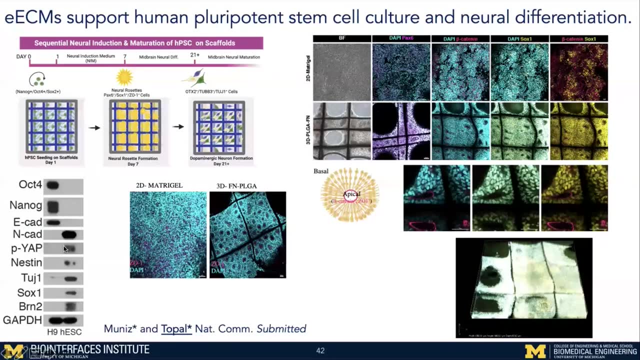 analysis of showing: yes, we are able to get this protein expression without differentiation. oh sorry, um, with the neural oops, with the neural differentiation. this is the. this is the part that we show. there is no differentiation of foreign, of for non-organic adherence there. all right, so what do we do here? this is: we call them eecm. um, they supporting hemoglobin stem cell. 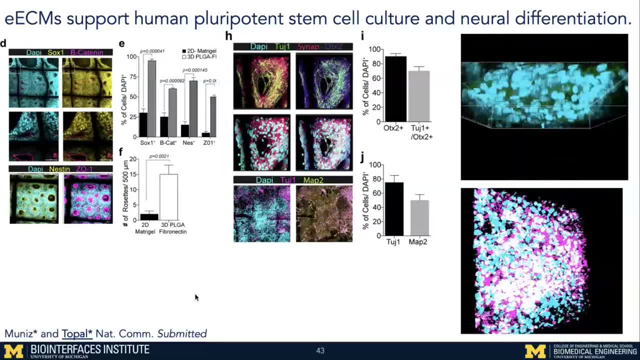 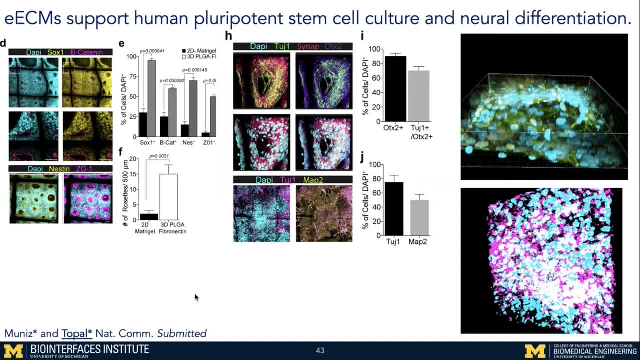 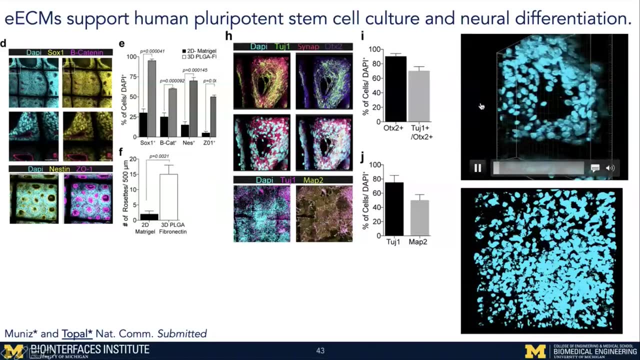 culture, neural differentiation. so at the beginning, like i mentioned earlier, we make the neural rosettes- beautiful rosettes, they're appearing here, and then we further um, investigate it. but we can make it neurons and you can see um here, maybe here too, uh, better images of these neurons, starting making it after 20, 25 days. 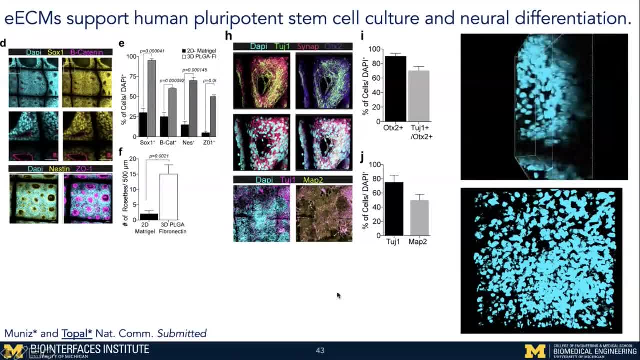 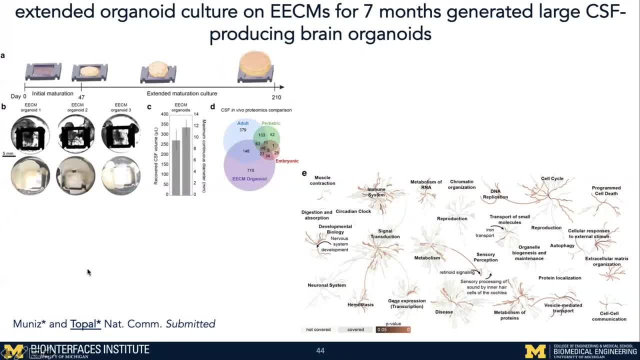 um all right. so later, um my, um the phd student, he for she forwarded, investigated uh to um expanding maturation up to seven months, and we get like a ball of it and we call them like eecm organates and she, she get a lot of single cell analysis. 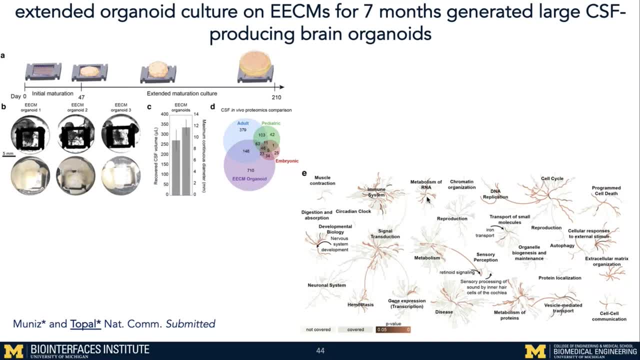 of that. i'm not showing it because the paper submitted, so i just wanted to show the images, part of this, so. but she was able to get like um, all these, um different part of uh differentiation and um neural system and homostasis, gene expression of transcription, blah, blah, blah. 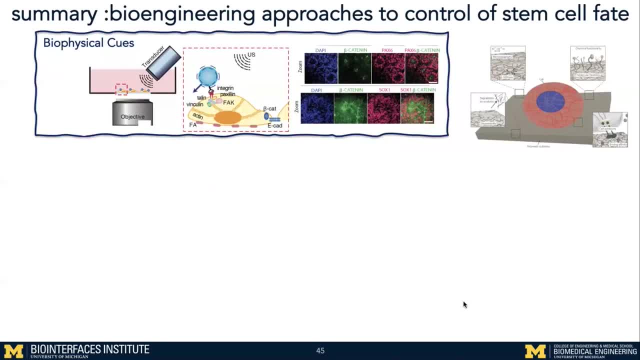 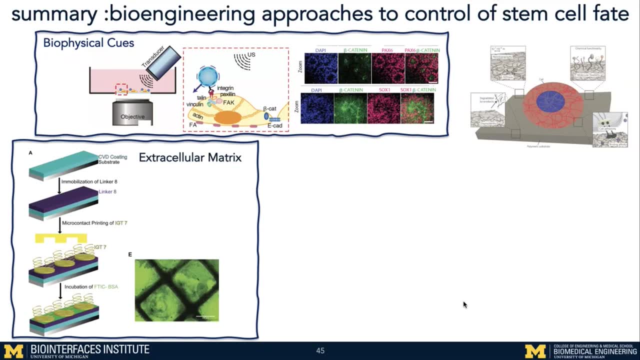 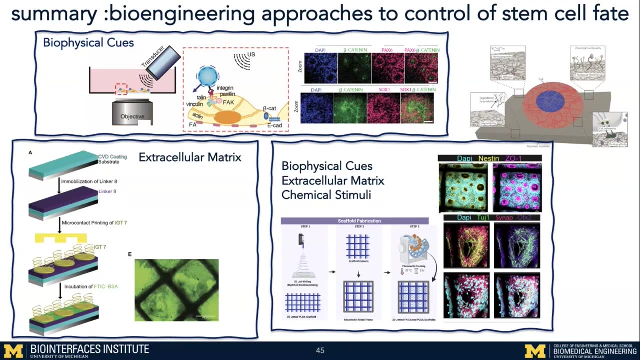 so with that um, i hope i was able to show you- all of you do- how biophysical cues is changing stem cell fate and using ssm metrics, how changing the stem cells and maintain poor policy and using all of these in one in the 3d cell culture. so, as a conclusion, the we can do it is: 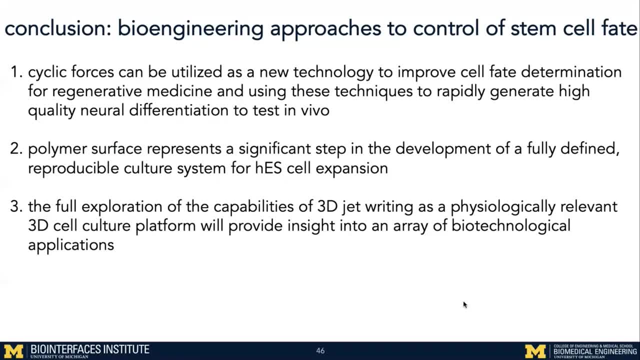 like by engineering approaches to control stem cell fate using cyclic forces, can utilize a new technology and we can use the polymer surface instead of using metrogel because, as you know, with the pandemic there is a metrogel shortage. i'm not sure whether you're aware of it, but now. 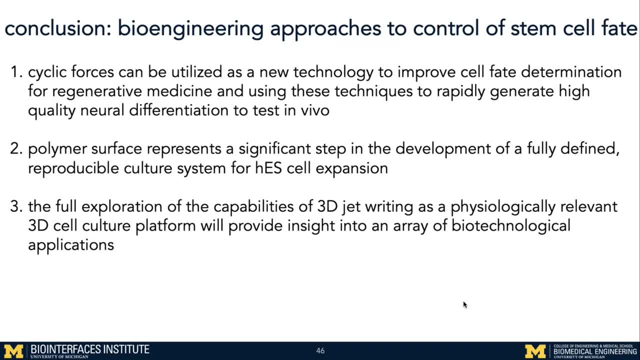 we need some polymer surfaces in order to supply and, at the same time, we don't need xanagenic material that introduced, or we don't need xanagenic material that introduced, or we don't need our cells, if you want these in our body. another thing is um the part. the last part is a 3d cell. 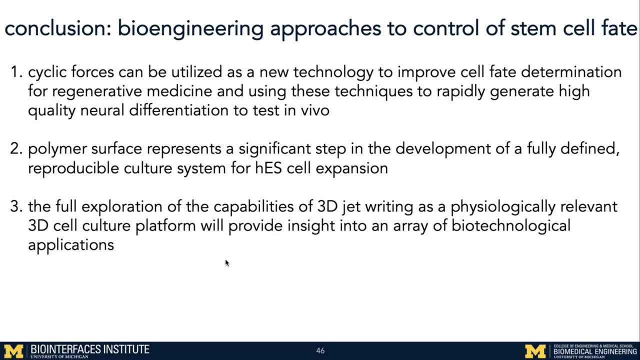 culture. we can use this to use as an array in the biotechnology application, the um, the idea. when i started this 3d um culture, the, the material. since this plga is a biodegradable, i wanted to use this as a like getting getting the patient cells getting in making pluripotent and depreciating 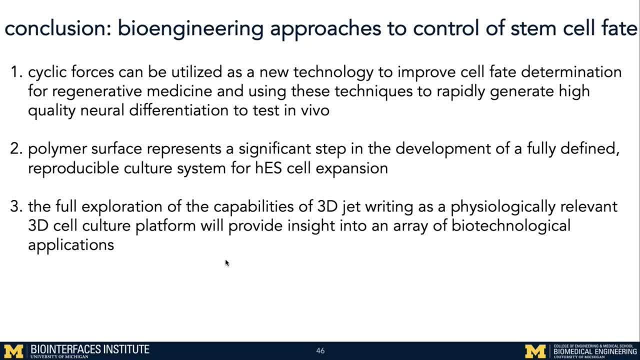 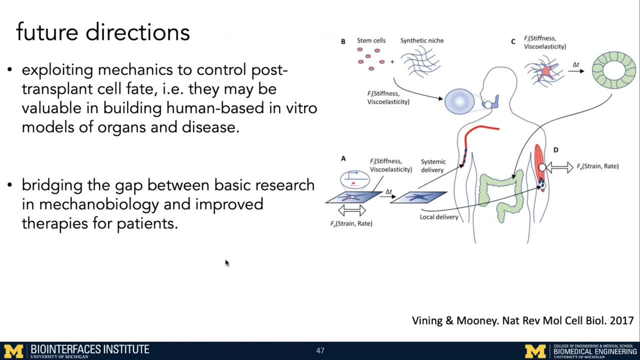 it- a neuron, in this case dopaminergic- and putting it back to the patient. so future directions can be exploiting mechanics to control post-transplant cell fate, um, for example, they may be valuable in building human-based initial models of organs and diseases. as you know, a lot of people are researchers that are working on these, and we can also bridge the gap between 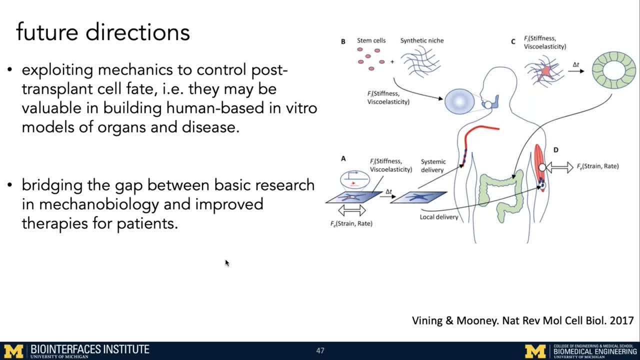 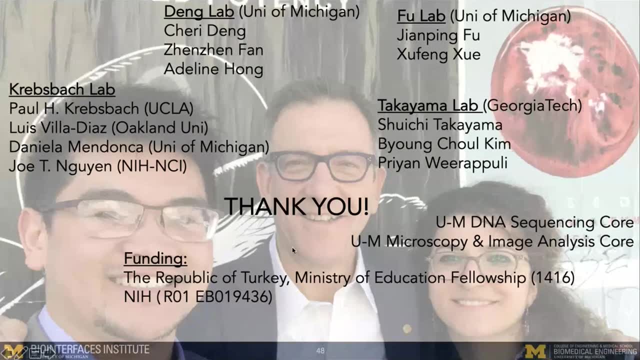 basic research and mechanobiology and interpreter piece for patients. so with that i would like to thank my api, paul krebsla- now he is the dean of the school of dentistry at the ucla- and, of course, my mentor and another mentor, oakland. krebsla is the dean of the school of dentistry at the ucla and, of course, my mentor and another mentor, oakland krebsla, is the dean of the school of dentistry at the ucla and, of course, my mentor and another mentor, oakland. 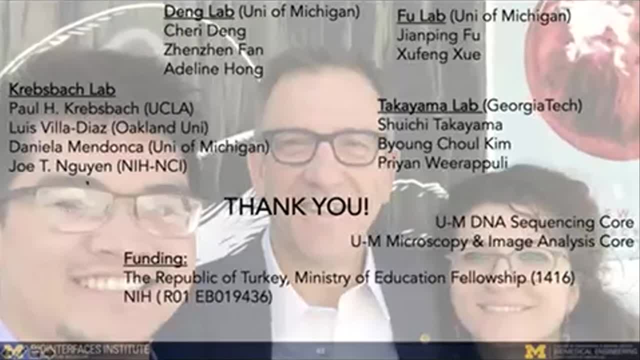 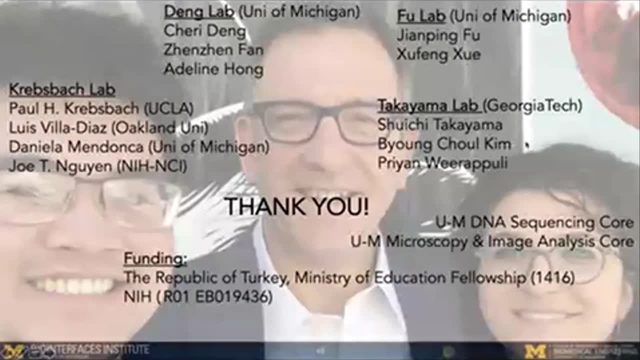 the university louisville and joe, my buddy, and now he's an nih nci, of course, full lab at dang lab, shiradang my professor and jumping through and shufang and take him a lot. oh, i didn't talk. talk about that part of the project with the um- microfluidics. i thought i wouldn't be able to. 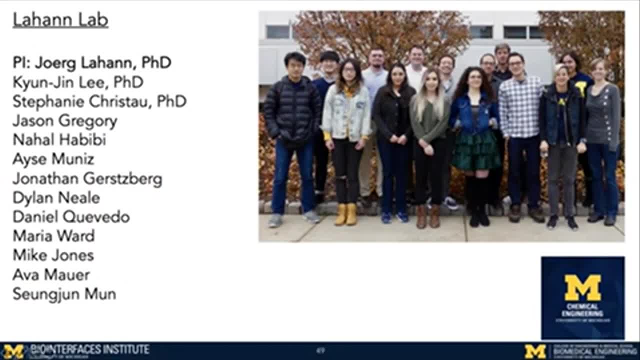 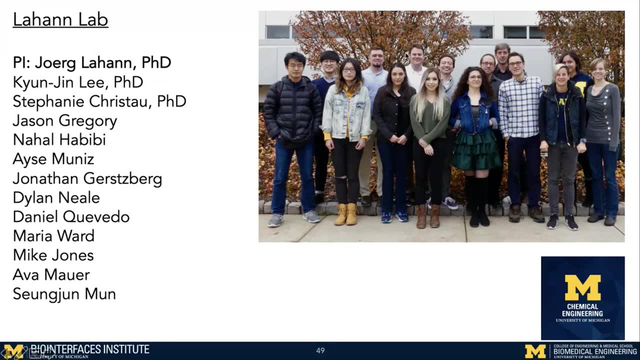 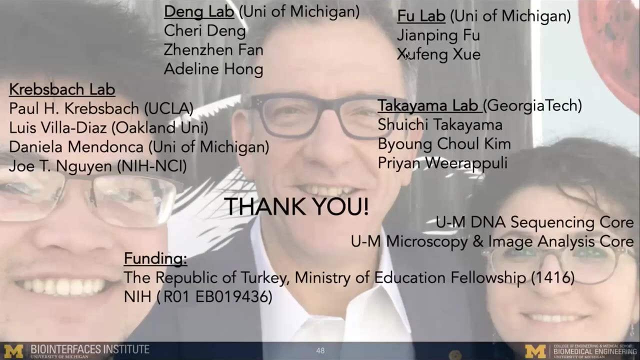 finish it and and other thing is um york lahan's group, here's york lahan and um all my friends and with that, yeah, so if you have any question, i would like to thank, i would like to take it. thank you, you and your doctor, thank you for your uh impressive presentation. 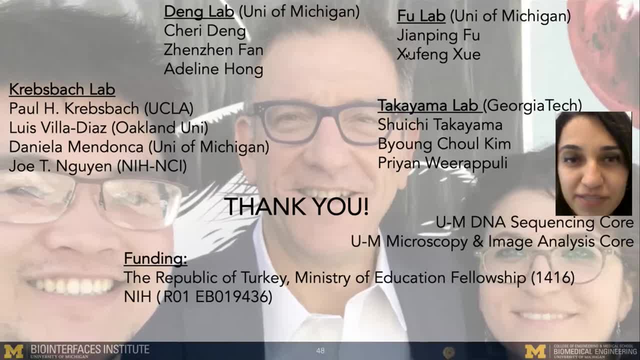 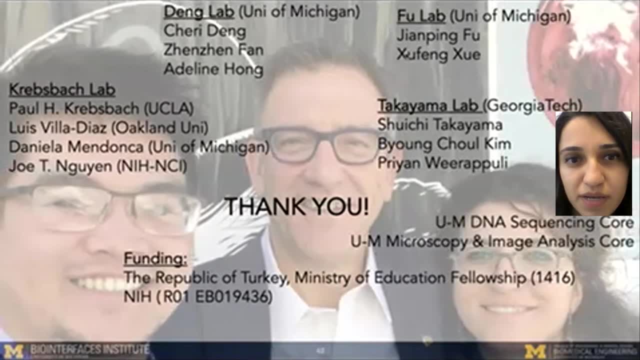 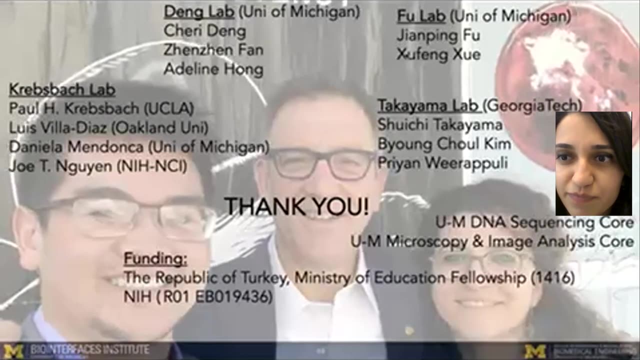 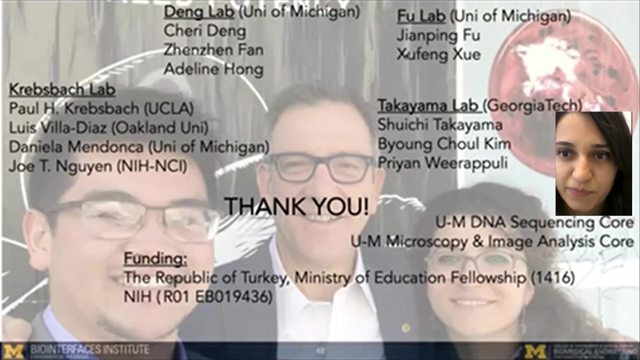 thank you, dear participant. if there is any questions about the presentation, please ask right now, and you could raise your hand to ask. uh, first of all, i would like to thank you very much, um, about our workplaces. you have offered us a very nice project, a few projects. thank you very much. 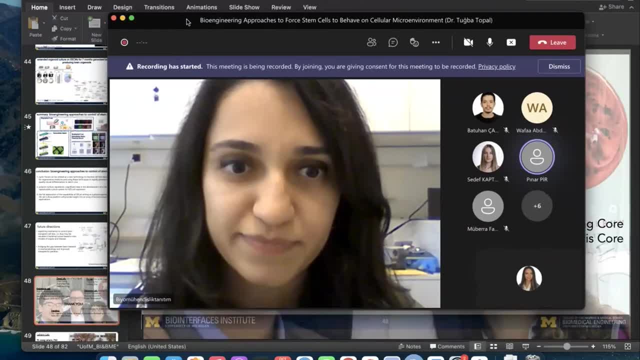 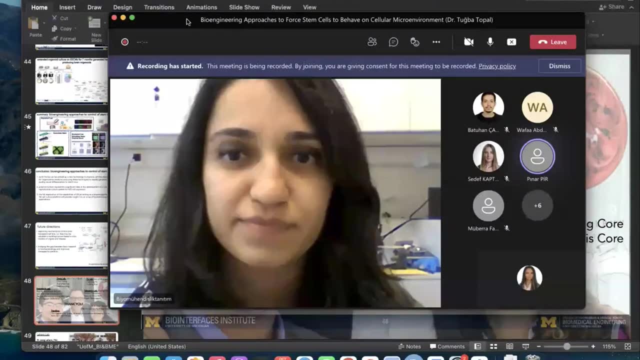 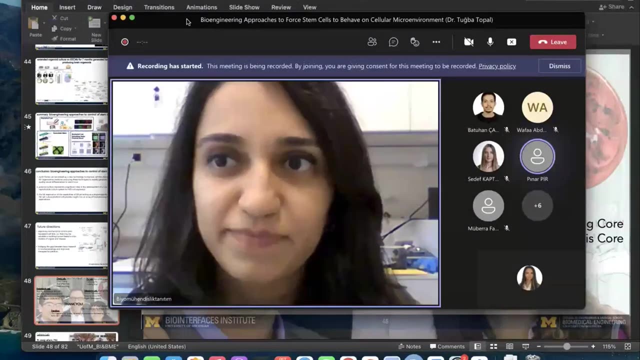 uh, i guess you are in turkey right now. uh, are you going to continue in turkey? yes, teacher, this, so if your workplaces uh will continue like this, uh can you organize your infrastructure? or do you have a search for infrastructure? because these are very high technology needs. these are very high technology needs. 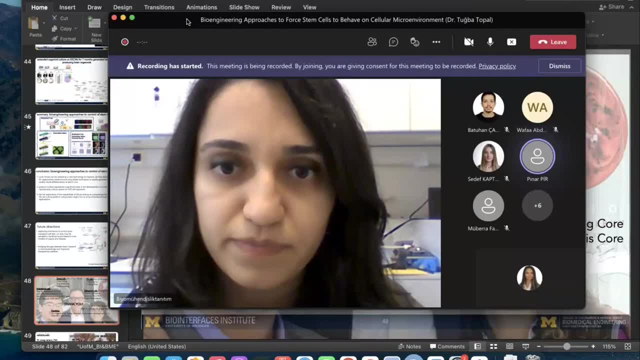 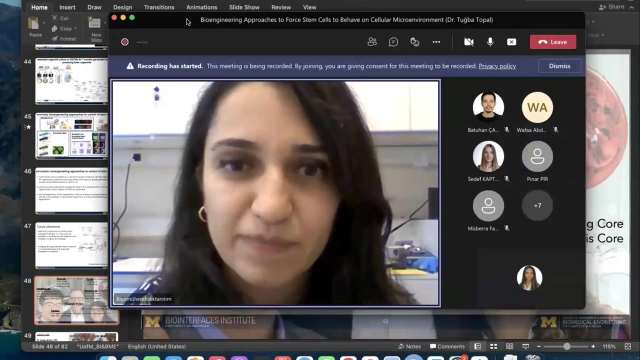 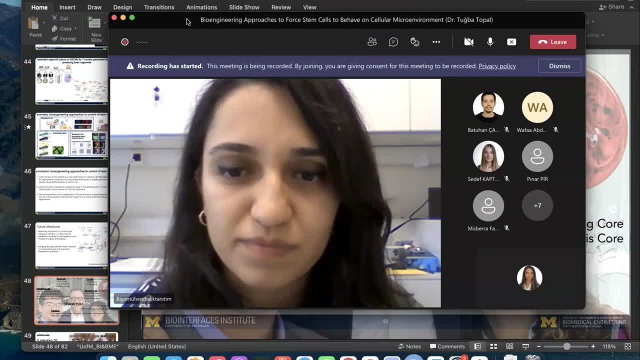 As you said, 3D printing is very expensive. It's not easy, but I'm not a kid right now, so I don't have the infrastructure to do it. Naturally, if there is a materialist who will collaborate in different universities with the infrastructure. 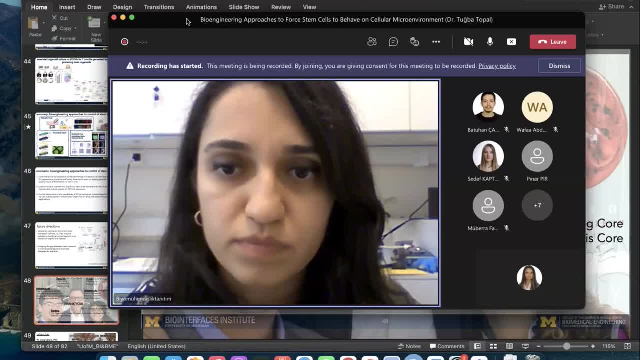 I think it's better to do something like this. I said this already, but I think it's better to go more on regenerative medicine, so I'm thinking of continuing that. I think it's better to go more on regenerative medicine, so I'm thinking of continuing that. 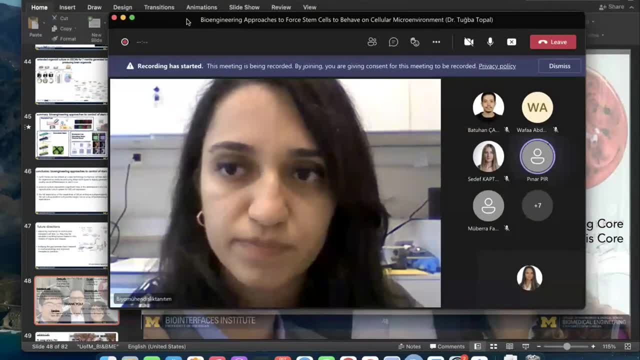 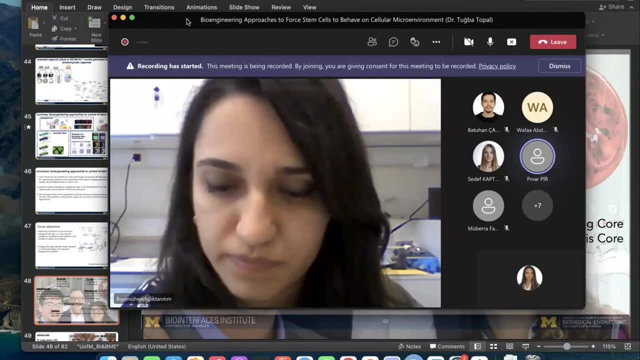 I think it's better to go more on regenerative medicine, so I'm thinking of continuing that. I don't know if I can answer your question. Yes, teacher, Frankly, as you said, it should be the same in Turkey. 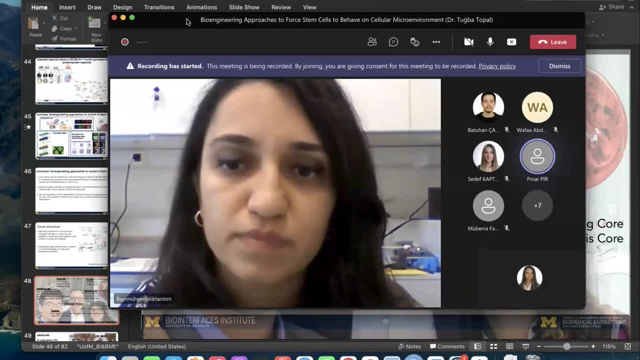 Because there is a cultural laboratory in one university, there is sequencing in the other. It is almost impossible to put them all together, But if you work collaboratively, in fact, there are pieces of infrastructure in Turkey. Is the cost of it now compared to TÜBİTAK? 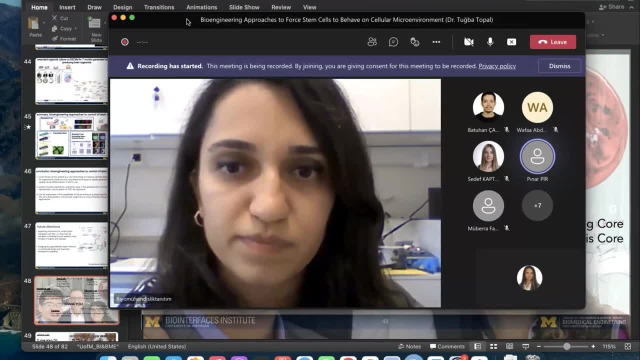 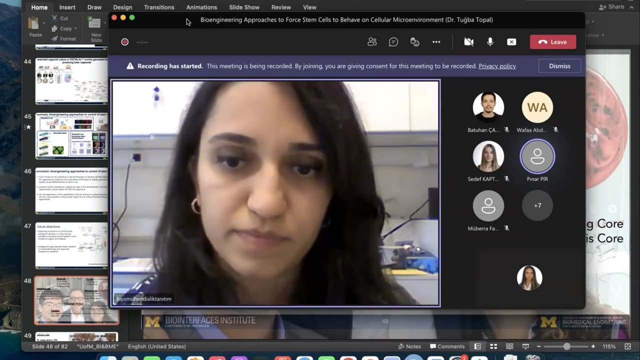 Or do you meet with the European Union and NIH projects? It is a difficult road. You will have to make a little more effort in Turkey. I hope you have felt it. I wish you good work. We have a lot of work in bioengineering, but I am working in bioinformatics. 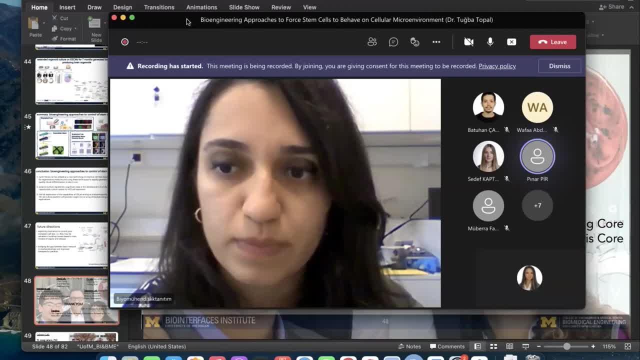 I am open to collaboration all the time. If you want, come and visit us, Let's meet, let's meet. I say We are waiting all the time. I thank you very much. I thank you. I don't have any other questions right now. 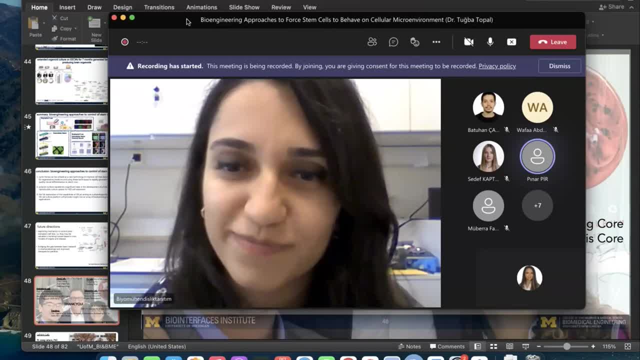 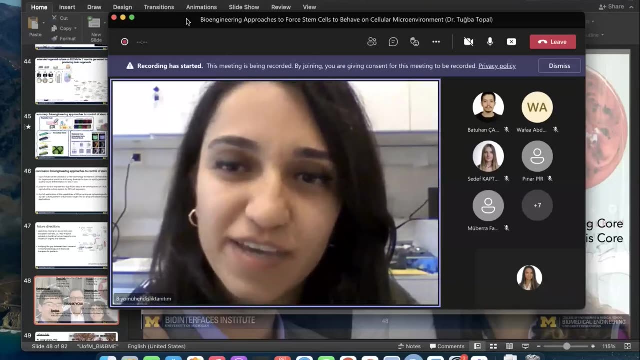 Thank you again. Thank you. If there are any other questions, I can take them. Teacher, actually I have a question. Come on, ask, Ask. What is the effect of the size and stability of these polymers and hydrogels in the use of matrix, in the use of root cells? 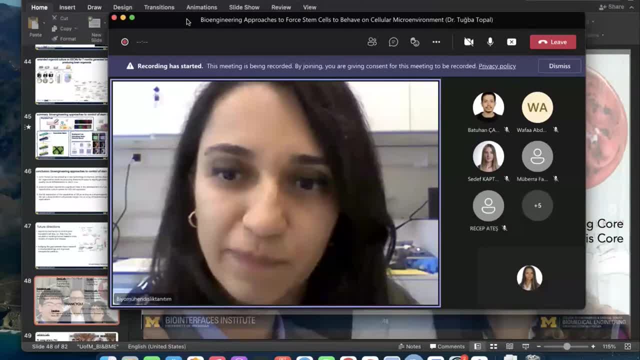 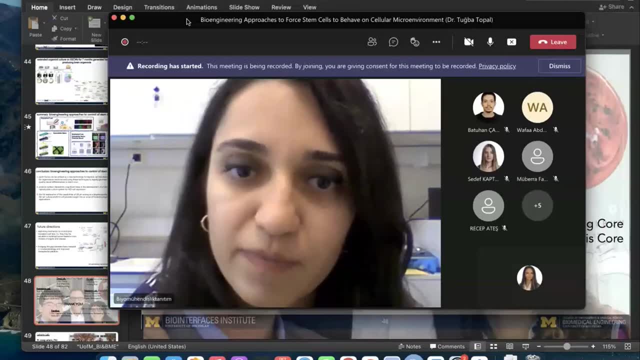 I mean you ask, I couldn't get your voice. teacher, Can you repeat At a certain temperature? you know, if you ask whether there is degradation in culture conditions, the polymer could stay there for up to 7 months. Then we didn't let it continue. 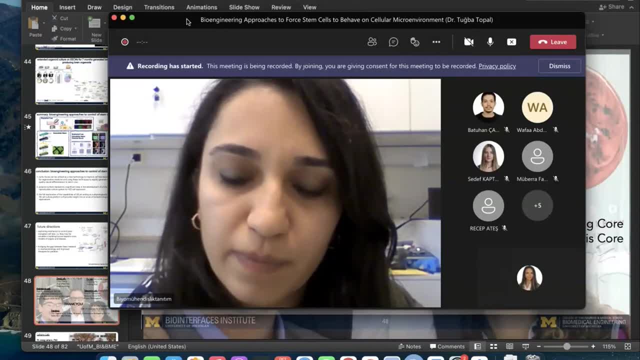 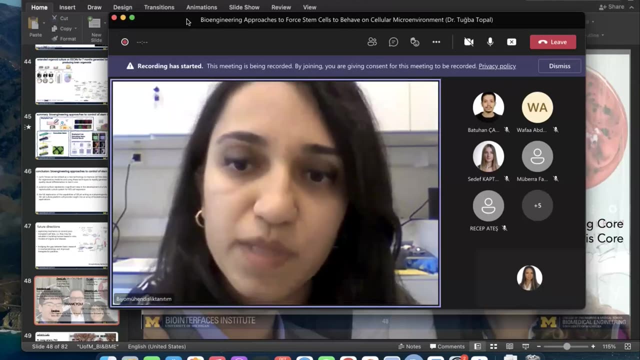 You know, something huge happened After that. I don't know what will happen, But normally when the material of PLGA enters the body it is easily absorbed and does not harm the body. But in the case of culture conditions we did not encounter such a thing. 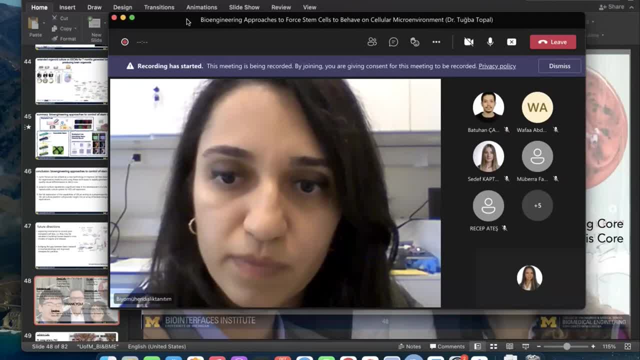 Because the body, you know, 37 degrees, But in the body of course it is more different, Because it just stands stationary, But in the body, for example. I will give an example. You know, in our section of University of Michigan, when I started, Scott Hollister had a trachea made of PLGA material. 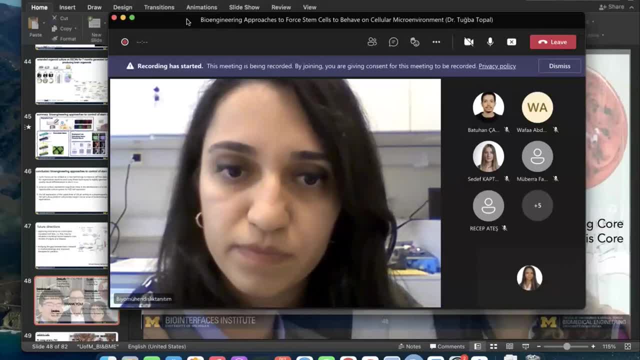 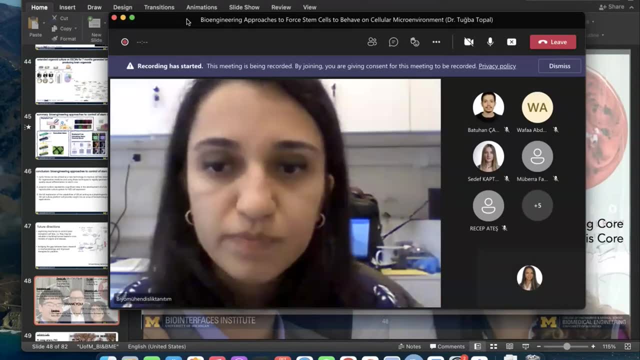 The trachea that they added to. the small child was born without trachea, For example. at that time, by slowly melting that PLGA there, it first formed a scaffold, then the body created it by itself, Because it doesn't stand as stationary in the body.